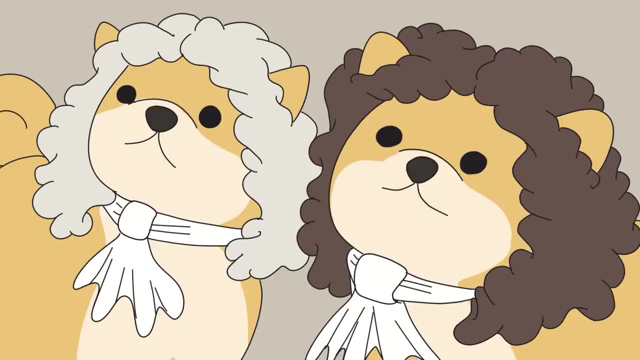 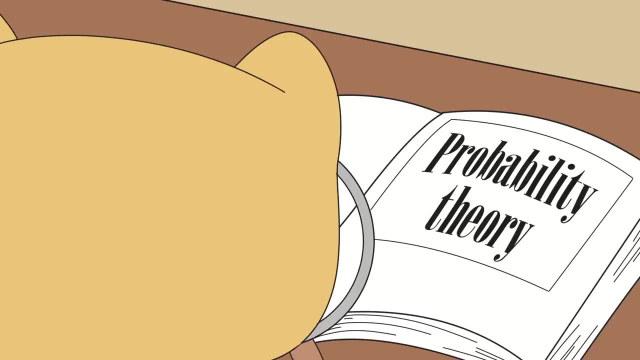 we can simply say: let us calculate without further ado to see who is right. Today we explore one approach to Leibniz's dream that uses probability theory to mathematicize truth-seeking. It doesn't take us all the way to that dream, but it covers some of 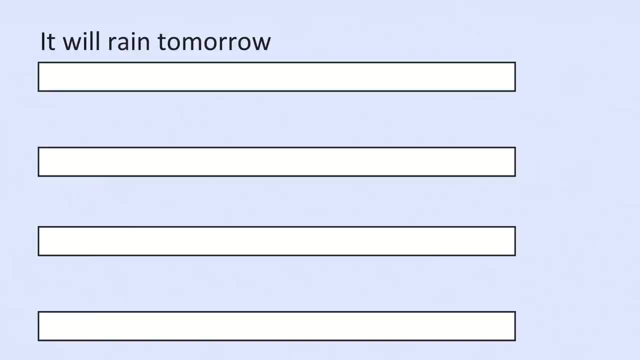 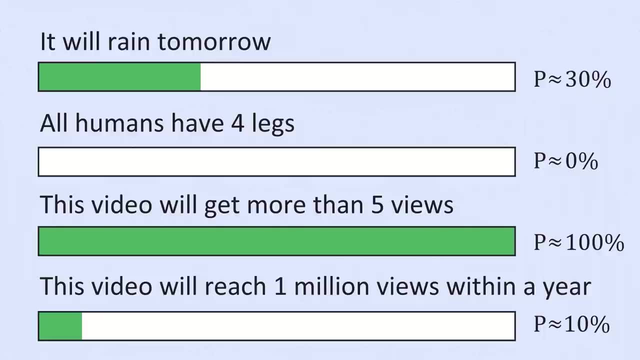 the ground. What we're talking about is Bayesianism. Its basic idea is that beliefs come with degrees of confidence and therefore we should interpret them as probabilities and not binary statements. Only having the statements x is true and x is false isn't enough to fully characterize a belief. 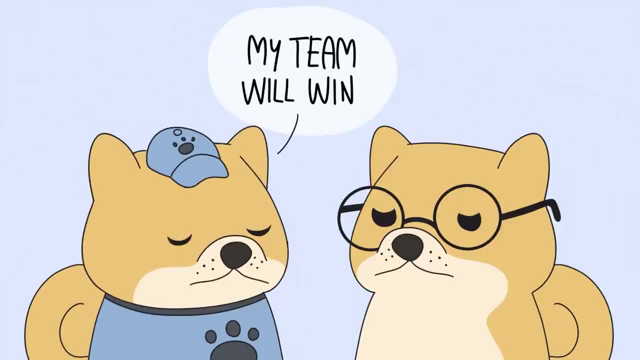 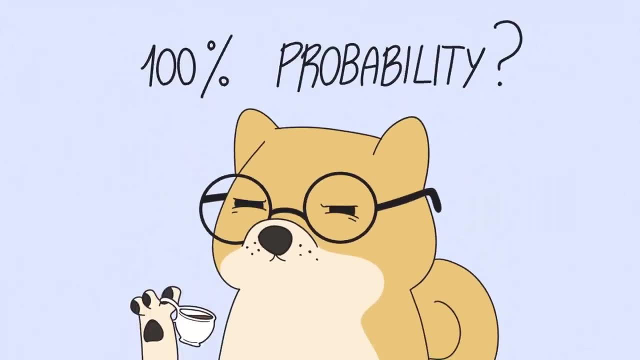 You'll often hear people say things like: I believe that my favorite sports team will win the game, But what does this statement actually mean? Does it mean they're absolutely sure? Would they be willing to bet money on the statement, And at what odds? And how can they update this vague? 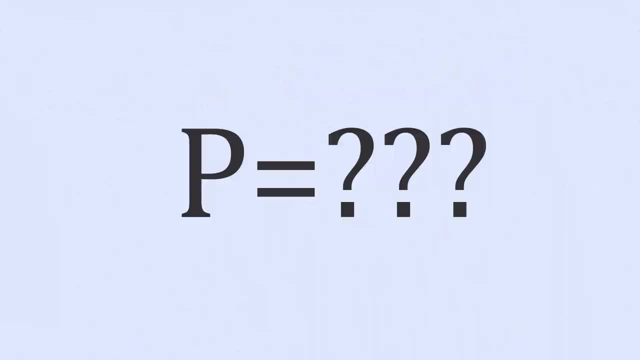 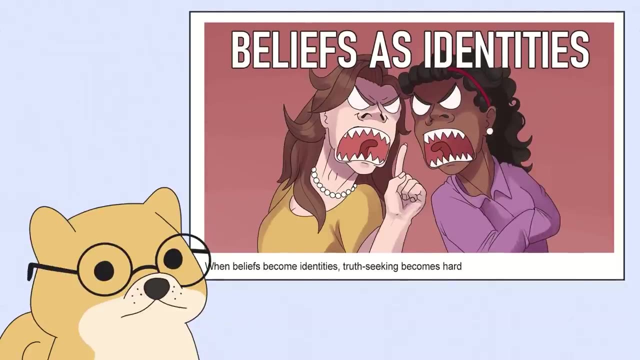 statement of belief when new evidence comes in Without reference to probabilities, common affirmations of beliefs can often be extremely vague. In their worst cases, people aren't even referring to a belief at all. They could just be cheering on their team. Bayesianism clarifies how. 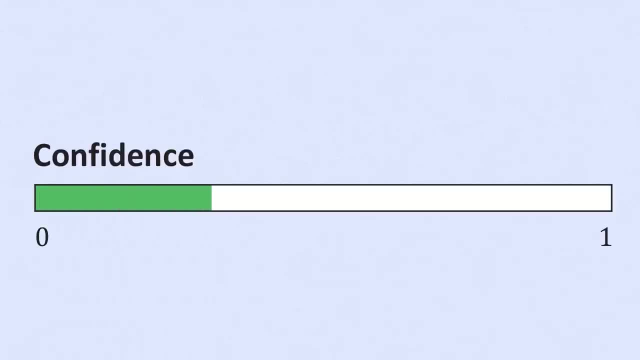 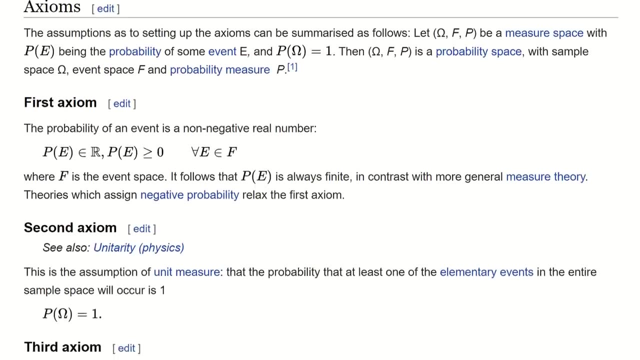 our beliefs should work. The probability representation, however, shows that we should have a degree of confidence in what we believe, represented by a number between 0 and 1.. The fact that beliefs are represented by probabilities means that they have to obey the axioms of probability theory. For example, beliefs can never add up to more than 1.. 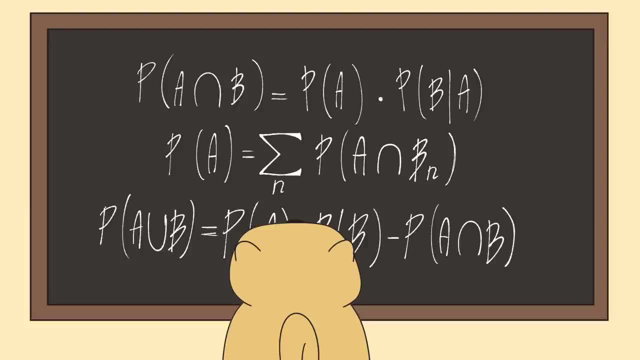 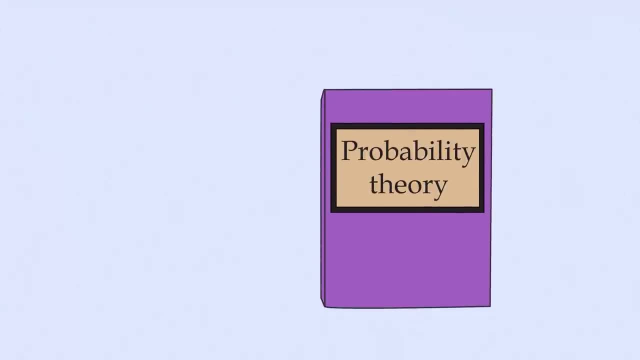 This also means that we can try to treat them formally and with quantitative rules, which gets us closer to Leibniz's dream. In fact, the most powerful consequence of this line of thinking is that probability theory gives us a formal way to update the level of confidence in our beliefs. 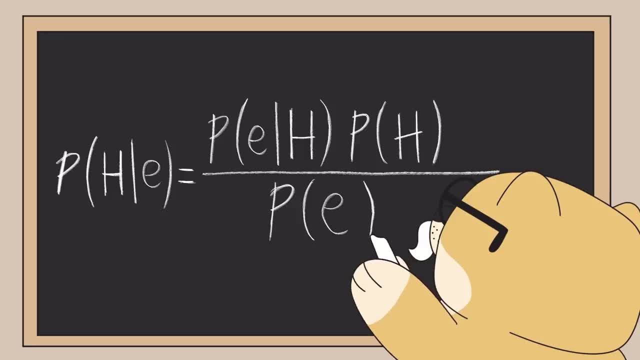 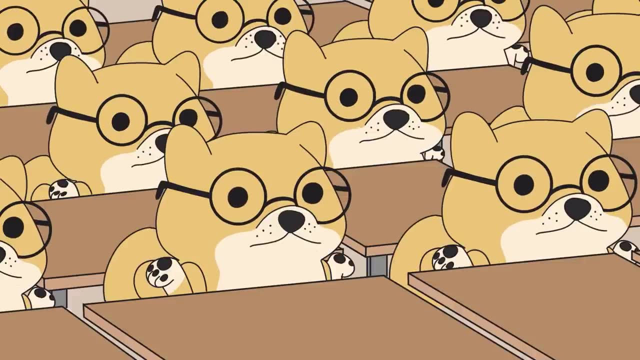 Bayes' Rule. Bayes' Rule is just a simple formula for the calculating conditional probability. If you ever took a class in statistics or probability theory, you might have come across Bayes' rule and thought nothing particular of it. But for Bayesians. 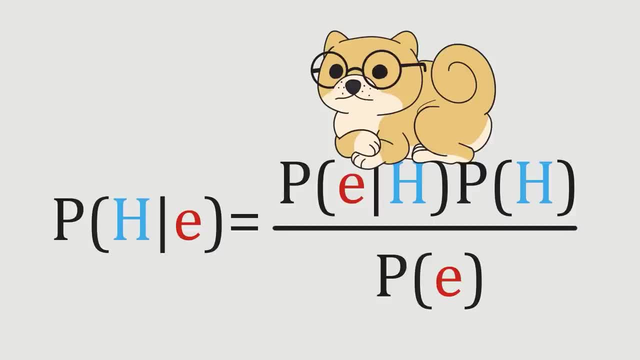 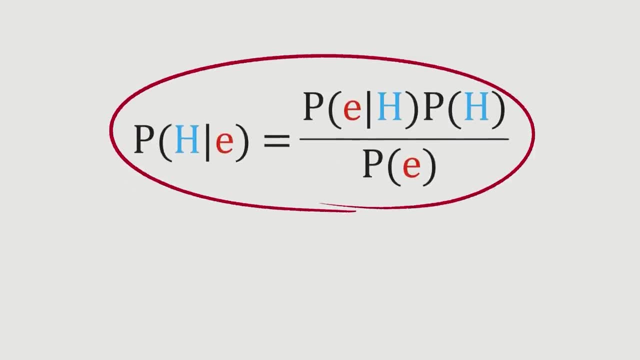 this formula takes on an additional meaning, forming the bedrock for how to change our minds in light of new information. It provides a systematic way of reasoning in terms of probabilities. It also has many important general consequences for the truth-seeking process. For example, we'll come to see how being open-minded can be informed by Bayes' rule. 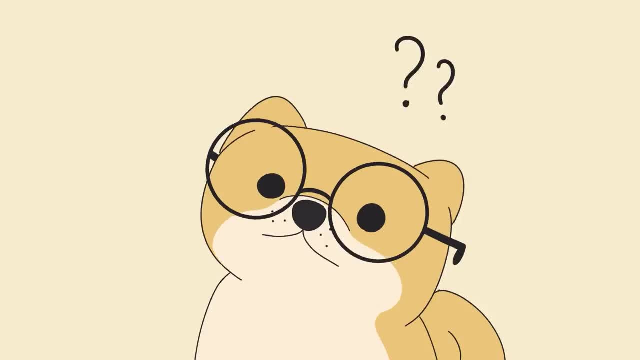 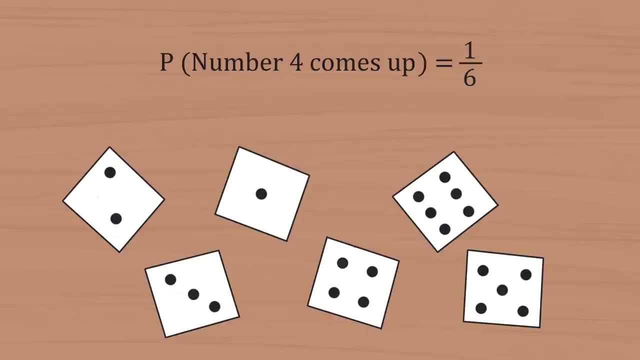 But before we introduce Bayes' rule you need to understand conditional probability. Suppose you want to know the probability that the number 4 will come up if you toss a die. The probability is 1 out of 6.. There is just one number, 4, written among the 6 faces of the die. Now suppose that you 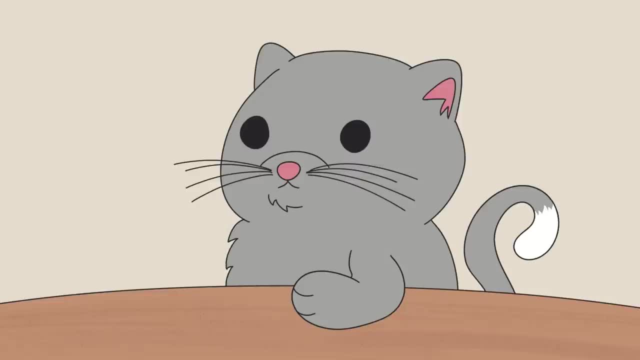 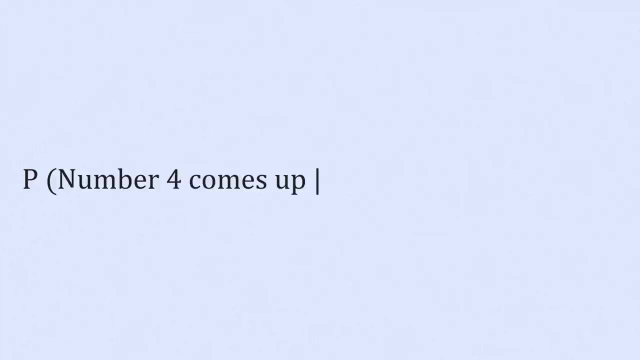 toss a die. but before you look at the result, a trusted friend tells you that an even number came up. Now you have additional information. What is the probability that the number 4 came up, given that I know that the result is an even number? There are just three possible even. 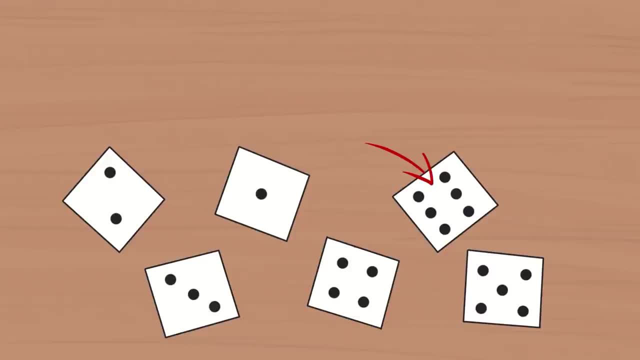 numbers that could have come up: 2,, 1, and 2.. 4 and 6.. Therefore, the probability that 4 came up, conditioned on the fact that the result is even, is 1 out of 3.. 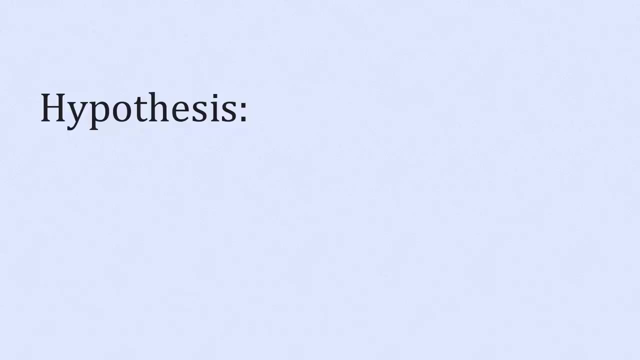 Now let's make this idea more abstract. Let's say we believe in some hypothesis, H, with some degree of confidence, which we represent with a probability Call that our prior probability in H. H could refer to anything we might believe about the world, such as: 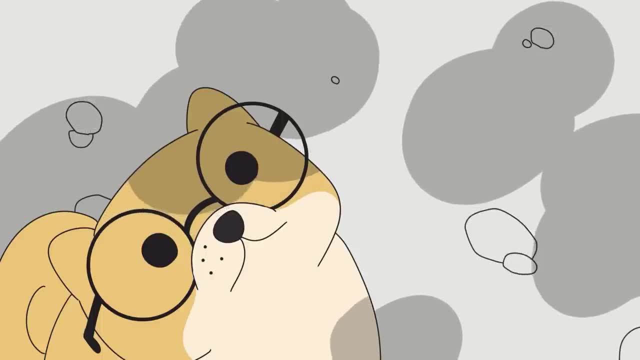 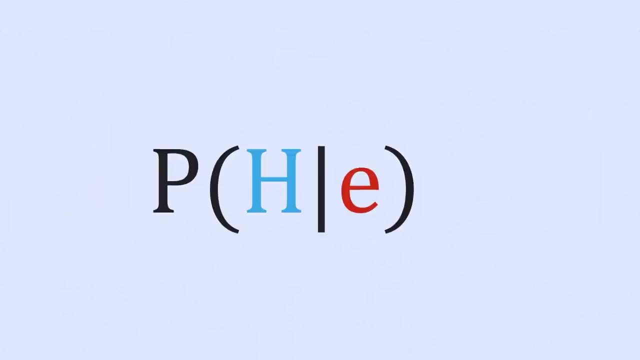 it's going to rain tomorrow. Then we observe some evidence- let's call it E- that influences our degree of belief in H. How do we update the probability of H given that we observe E? Bayes' theorem clarifies this. It was easy to do in the case of our hypothesis being 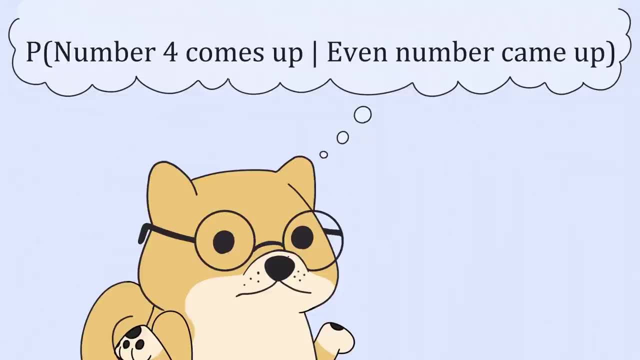 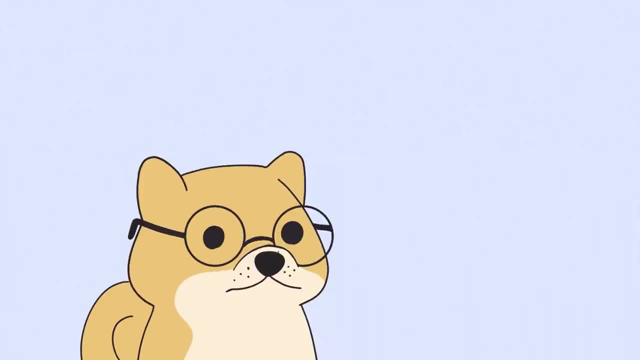 the result of tossing the die is 4, and our evidence being the result of the die toss is even. But it's not always this simple. You'll want to calculate conditional probabilities in more interesting cases. Let's consider another example. You're in the middle of the summer. 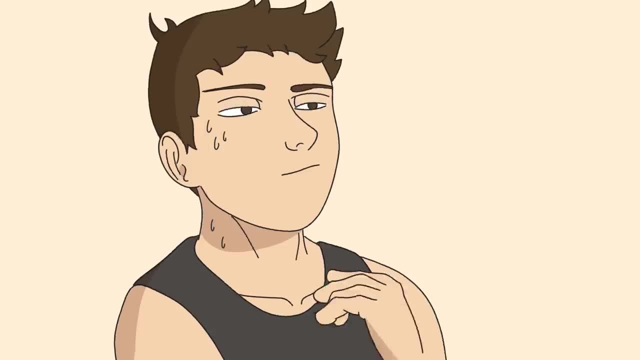 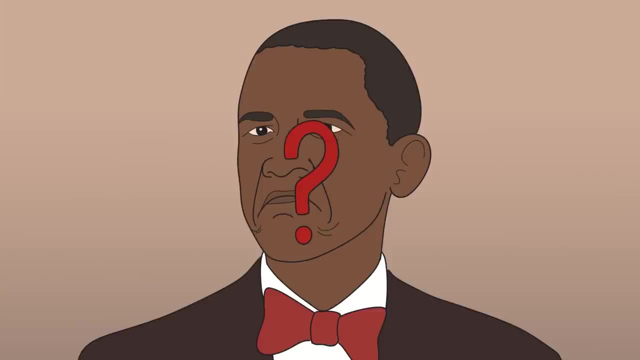 but your friend complains that he's having the chills. Immediately, a hypothesis shows up in your mind: It might be the flu. To you it seems like a reasonable hypothesis. But why is it reasonable, mathematically speaking? And what do we mean by reasonable? Well, it's not just a. 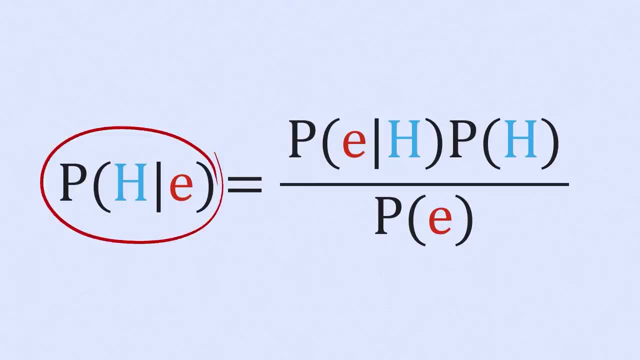 reasonable. anyway, Here we have Bayes' rule. On the left-hand side, the probability P of H, given E, represents our probability estimate of a hypothesis H, given the evidence provided by observing E. For us it will represent the probability that our friend has the flu. 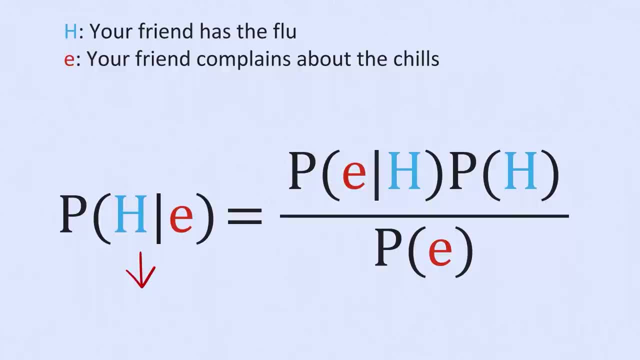 given that he is complaining about the chills. This is also called the posterior probability of the hypothesis. Now let's focus on the right-hand side. A key insight from Bayes' rule is that we can calculate the probability of a hypothesis, given the evidence, using the inverse. 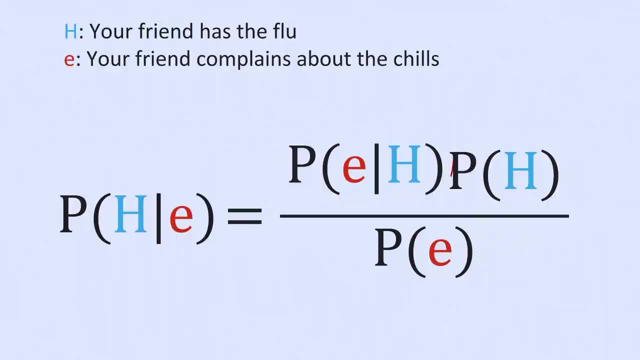 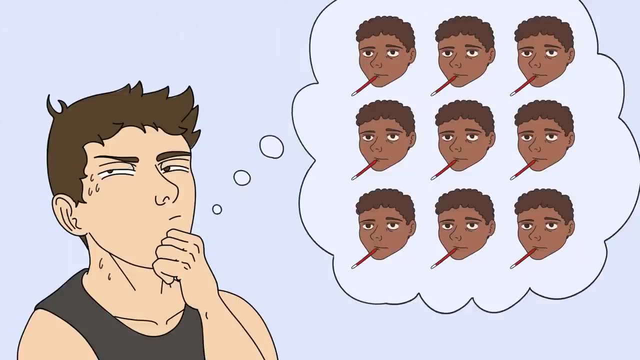 statement, the probability of the evidence. given the hypothesis. What this term of the equation asks us to consider is: pretend that you know that your friend has the flu, but that you haven't talked to him yet. Then how likely is he to complain that he has the chills? In other words, this term 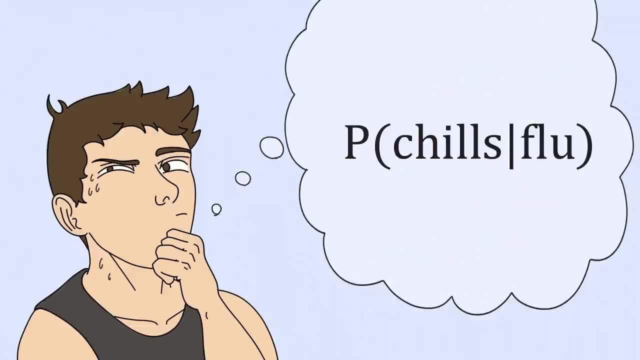 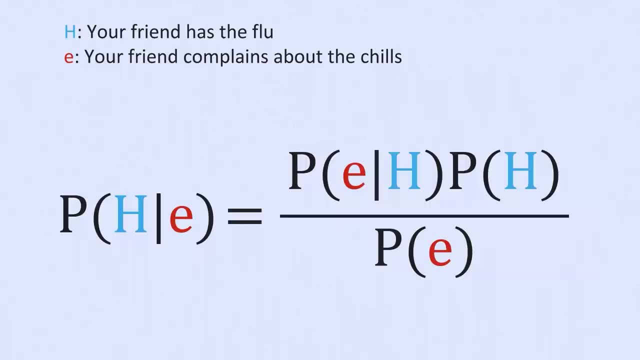 asks you to consider how likely the chills are made by the flu. The fact that you're now observing that your friend is complaining about the chills has to be ignored. Otherwise this term would always be 100%. Note that the term P of E conditioned on H is also called the likelihood. 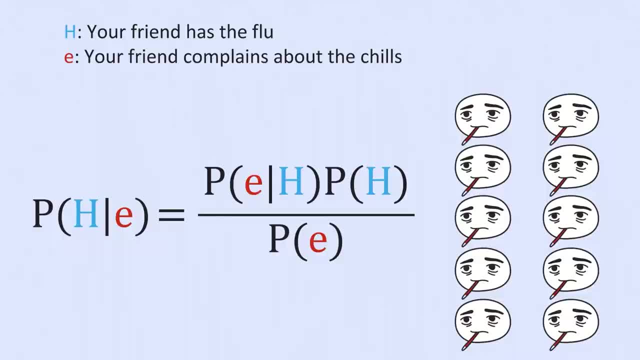 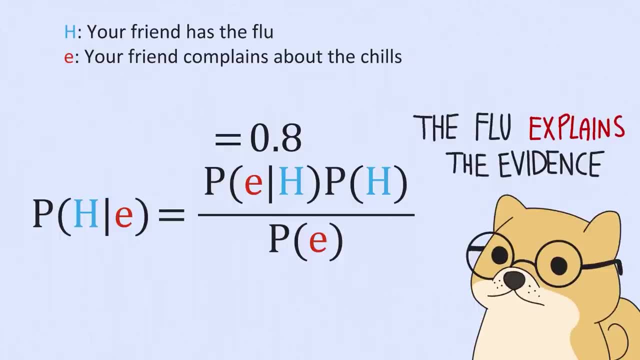 We'll use this word in the rest of the video. Now let's look at the probability of a flu. Now suppose that you read somewhere that 80% of the population complains about having the chills when they have the flu. You could say, although a bit vaguely, that the flu explains the evidence. 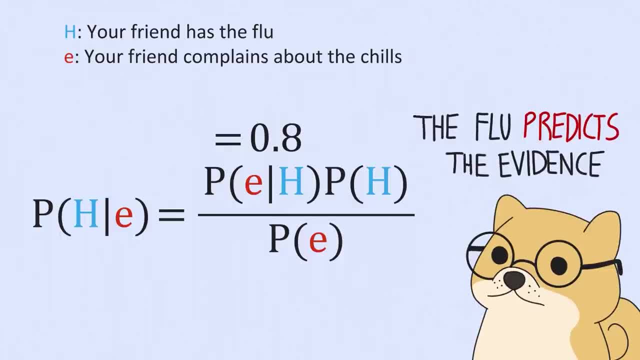 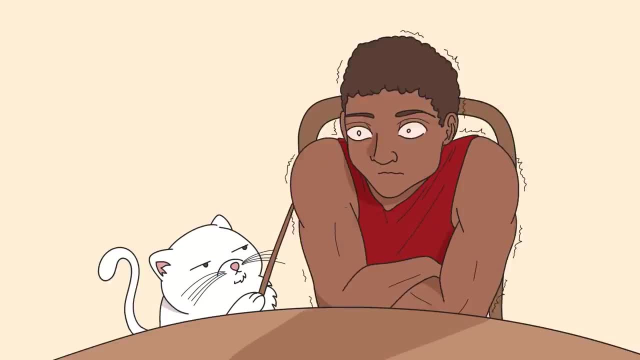 at hand. You could also say that it fits the evidence or that it predicts it. But now let's consider another hypothesis. Maybe your friend has met the chill cat, a magical cat that gives people the chills 100% of the time. This hypothesis fits the evidence even better because every single 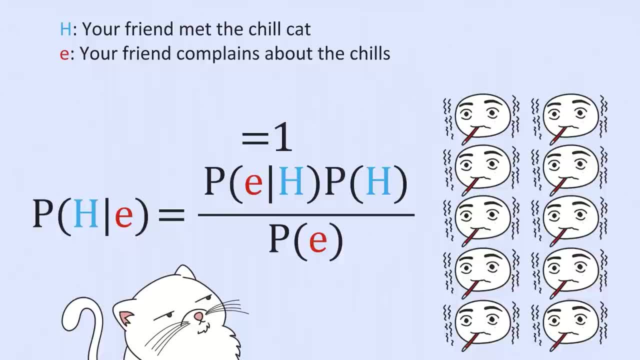 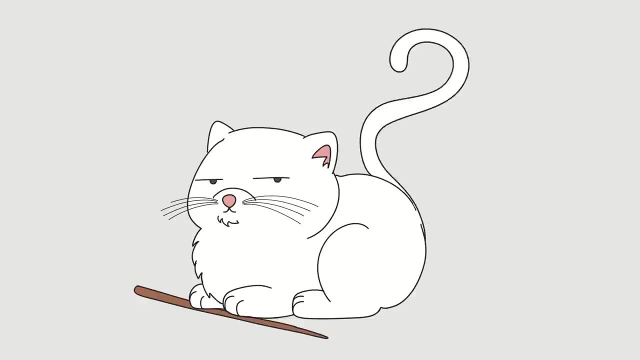 time someone's met the chill cat, they complain about the chills. Therefore, the probability of someone complaining about the chills, given that he met the chill cat, is basically 100%. And yet this hypothesis is clearly false. I never heard of such a cat. In fact, I just made it up. 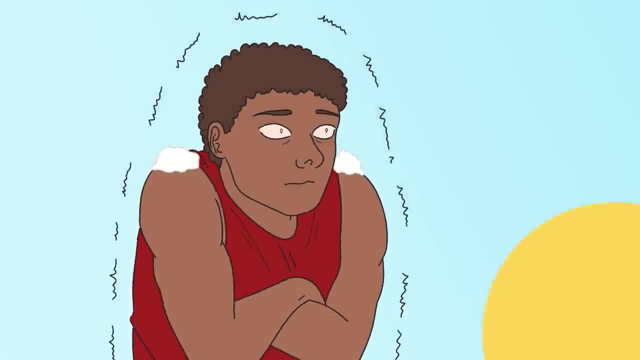 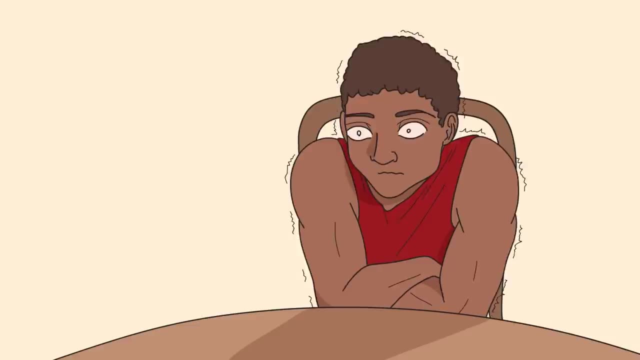 Or maybe your friend is shivering because the temperature is low, Except this can't be because it's a hot summer. This brings us to the next term of the equation, the prior probability of the hypothesis. This term expresses your degree of belief about H before encountering the evidence. 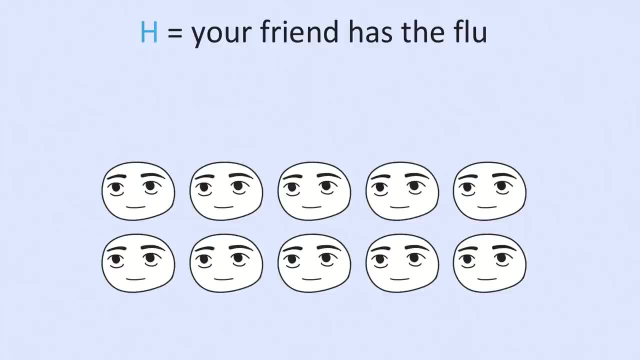 at hand. If H is your friend has the flu, you might set P of H to be the fraction of the population who have the flu at hand. If H is your friend has the flu, you might set P of H to be the fraction of the population who have the flu at hand. 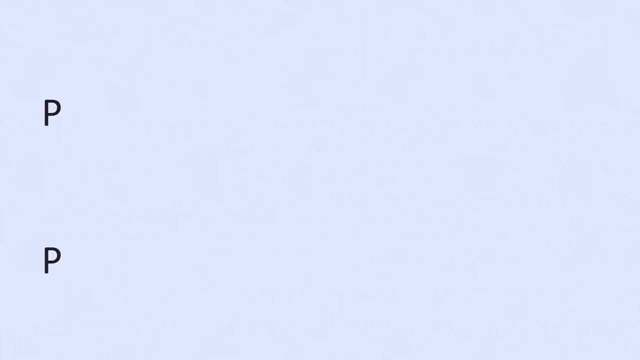 If H is your friend has the flu, you might set P of H to be the fraction of the population who have the flu at hand. Let's say that it's 10%. But now let's see what the prior probabilities of your friend met the chill cat and the temperature is low are. The answer is basically zero. 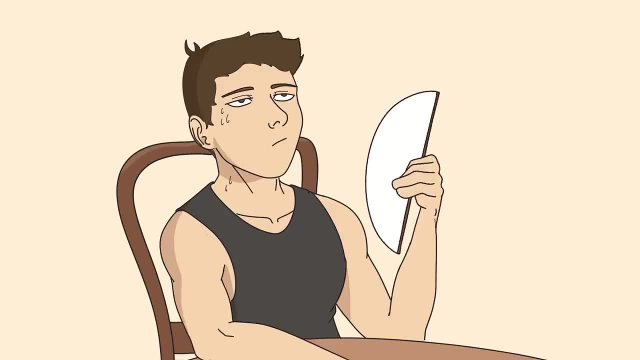 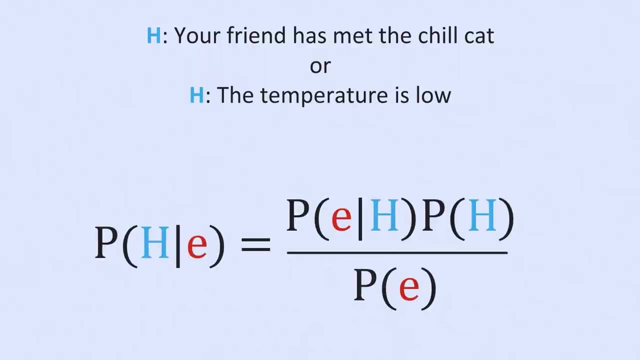 Zero people out of eight billion have met the chill cat, and the probability that the temperature is low has already been updated to near zero by the evidence that you're in a hot summer. These two alternative hypotheses sound unreasonable because, even if their likelihood is close to 100%, 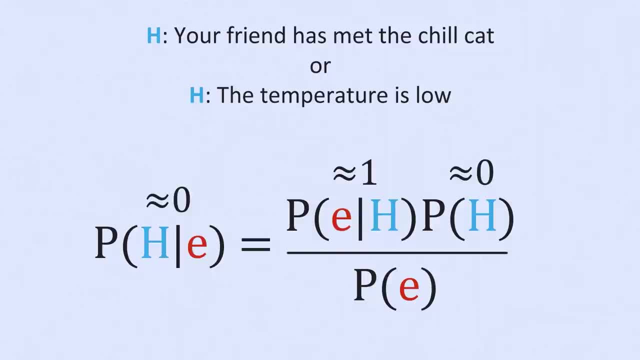 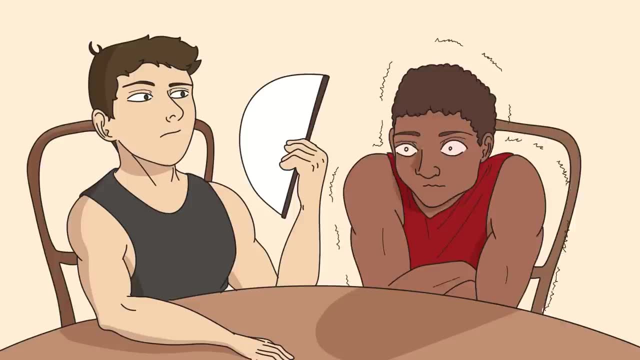 it's multiplied by a prior that is negligible and therefore their posterior probabilities get squashed. Now let's consider the denominator P of E. It is the probability of the evidence. Again, this is not the probability of the evidence after observing it. 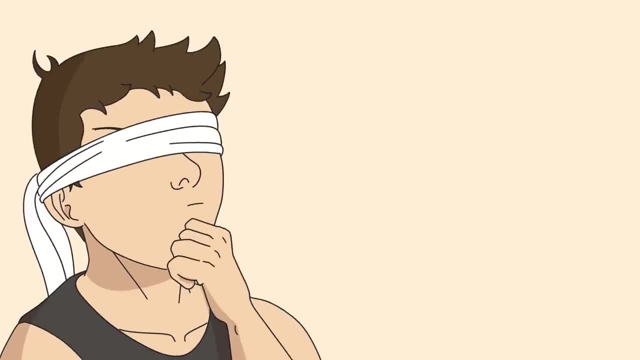 otherwise it would be about 100%. You should interpret P of E as asking: what is the probability that we would have given to the proposition that we would observe this evidence if we were asked prior to actually observing it? In our example, the answer might: 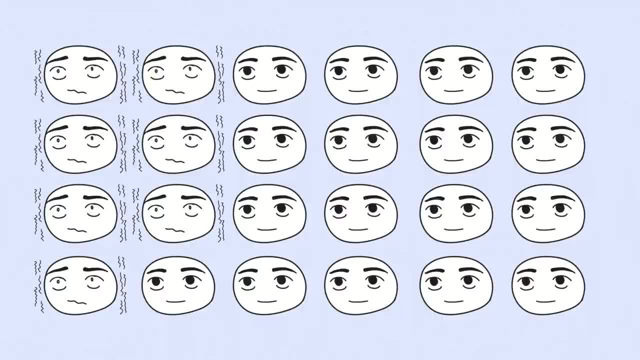 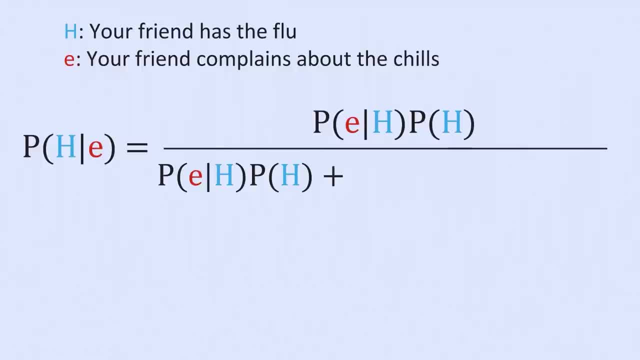 be the proportion of people complaining about the chills at this time of year. To gain intuition about this term, you need to decompose it into a sum: The likelihood of the hypothesis multiplied by its prior, plus the likelihood of the negated hypothesis multiplied by its prior. 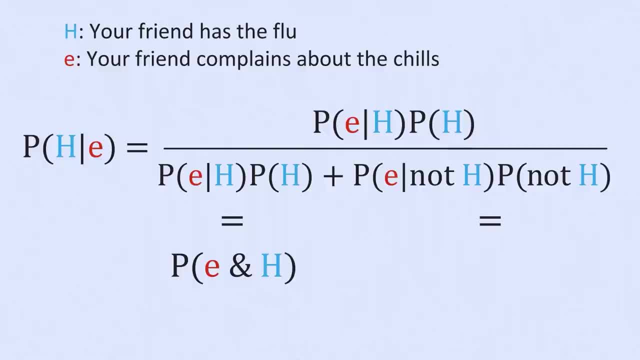 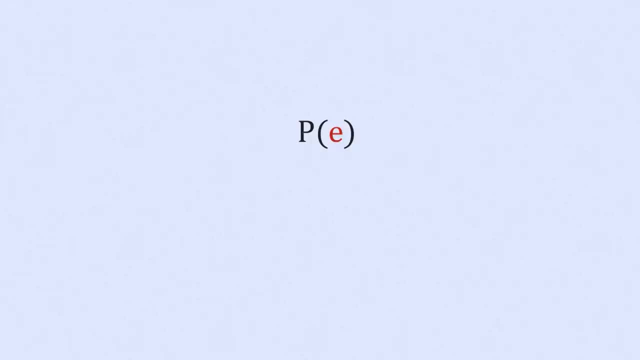 You should note that these two terms also mean the probability that your friend has both the chills and the flu, and the probability that your friend has the chills but doesn't have the flu. To see intuitively why P of E can be decomposed in this way, you can reason like this: 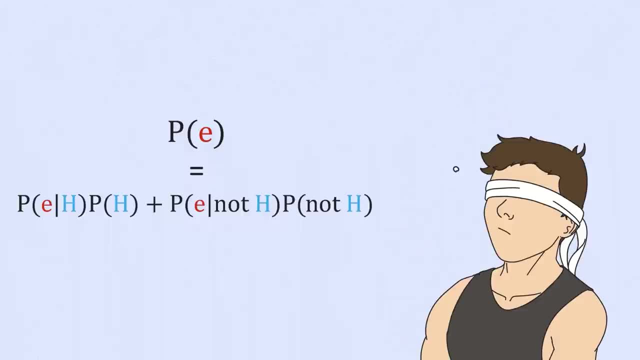 What you want to know is the probability that someone complains about the chills before you observe whether they really have the flu. Therefore, you might reason: well, the probability that they complain about the chills depends on if they have the flu or not. 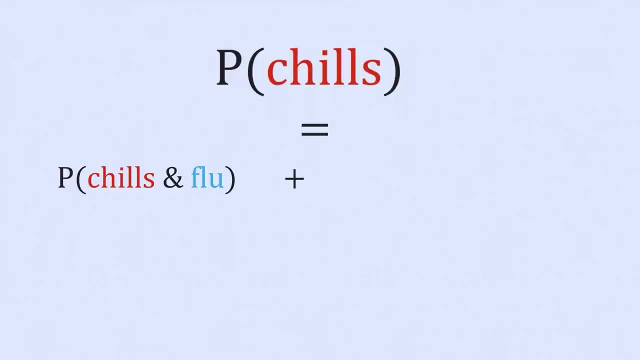 So you calculate separately the probability that they complain about the chills while they have the flu and the probability that they complain about the chills while not having the flu. Note that doing a simple addition works because H and not H are mutually exclusive. 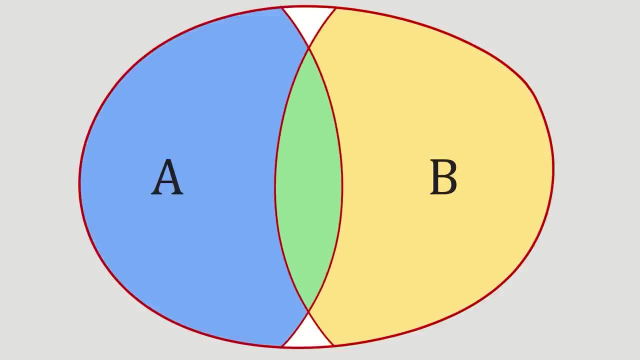 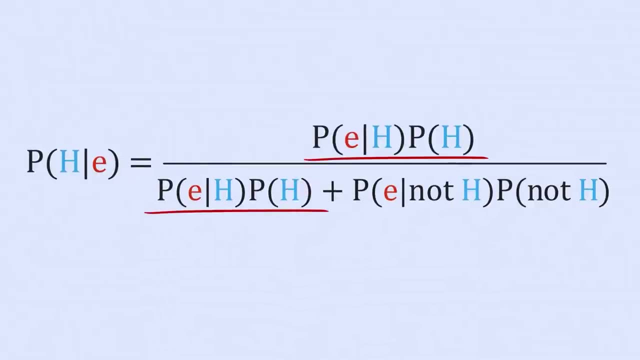 and they cover all the possibilities. Otherwise this decomposition would be slightly more complicated. Now back to Bayes' formula. As you can see, the first term of the denominator is now the same as the numerator. The second term has the same structure as the numerator. 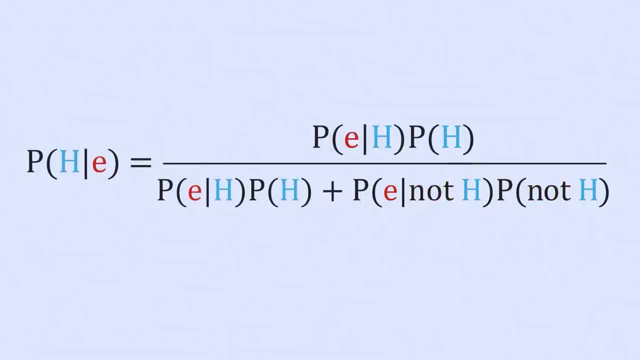 but it has not. H instead of H. This second term can drive our intuitions about the denominator. In the case of our example, it indicates how much not having the flu also fits the evidence of complaining about the chills multiplied by the prior. 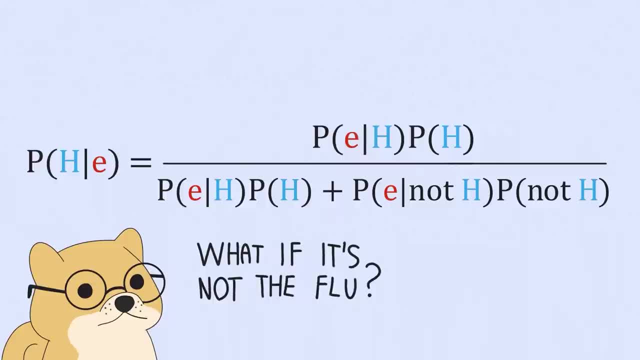 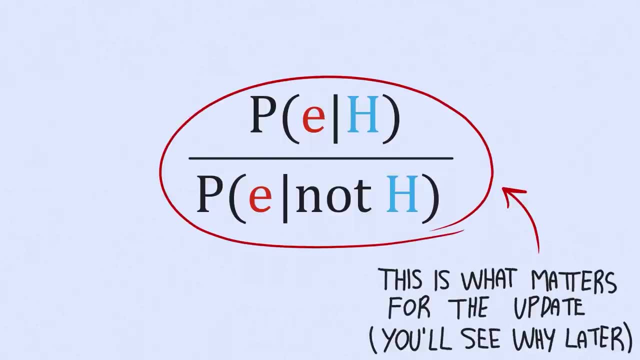 probability of not having the flu. You can see this term as considering the alternative hypothesis. The strength and the sign of a Bayesian update depends on how good your hypothesis is compared to the alternatives, not how good it is in a vacuum, In fact. 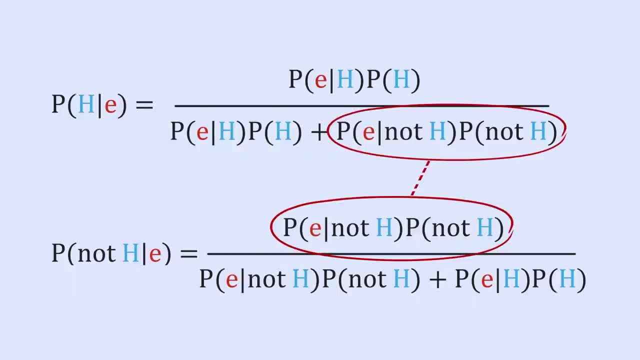 this term is exactly the numerator of the Bayesian update for your hypothesis negated. The higher the posterior probability of the negated hypothesis, the lower the posterior probability of the negative hypothesis. The lower the posterior probability of your hypothesis. We'll also see that if the likelihood of the hypothesis 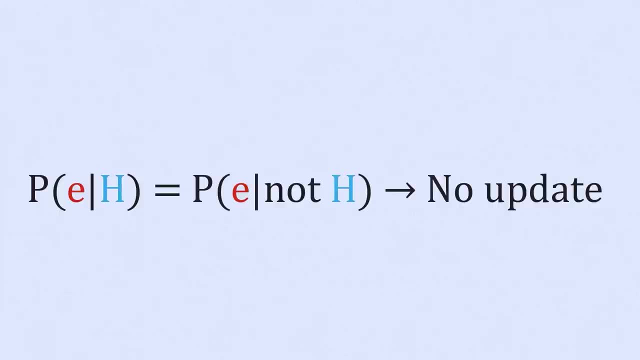 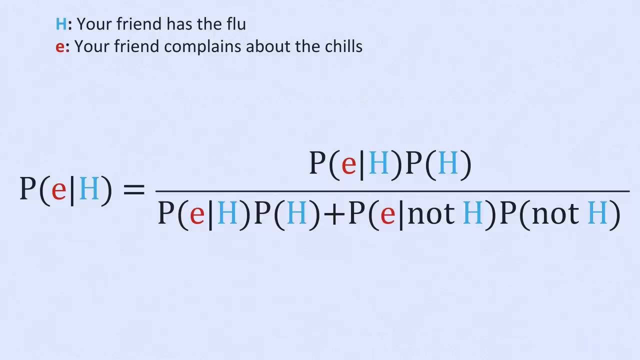 is the same as the likelihood of the negated hypothesis. there is no update. If your hypothesis fits the evidence at hand as well as the alternative, then it doesn't gain or lose credence. Let's plug in the numbers now. We said that, given the flu, 80% of the population complain of having 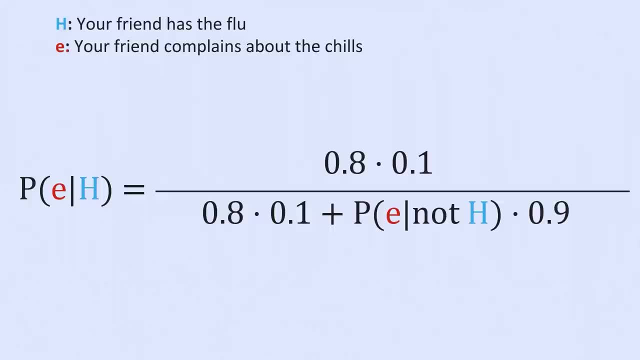 the chills. The prior probability of the flu is 10%, and let's say that, without the flu, 1% of the population will complain about chills anyway, because… I don't know, these are made-up numbers. Then the probability of your friend having the flu, given that he's complaining about the chills. 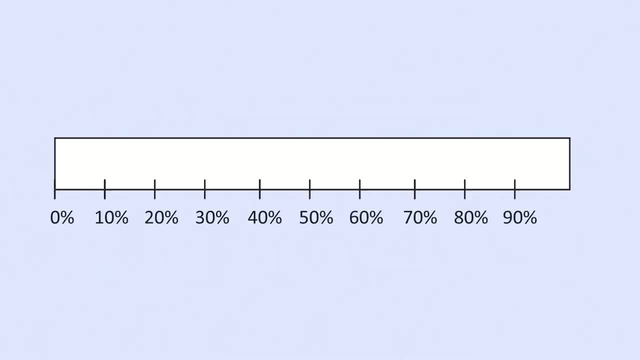 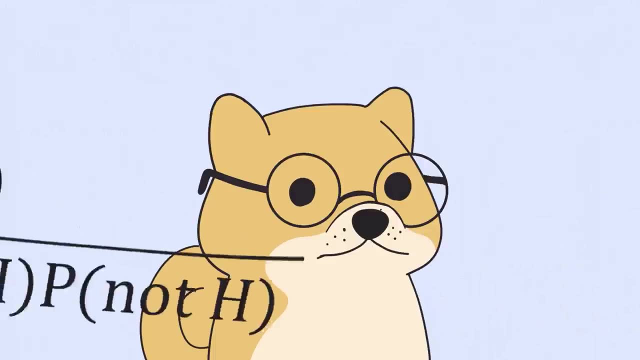 is around 90%, From a prior of 10%. after seeing the evidence, we updated our hypothesis to a probability of 90%. Now you might have formed some intuition for the formula. Maybe you see the meaning of each term and even that they embody rules of reasoning that aren't that. 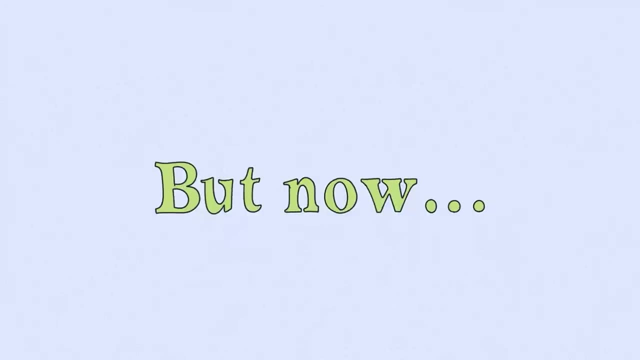 distant from how we might reason in day-to-day life. But this is probably not sufficient to see Bayes' rule clearly, so here's another explanation that could give you more clarity. Let's say that 20% of the population has the flu at this time of year. 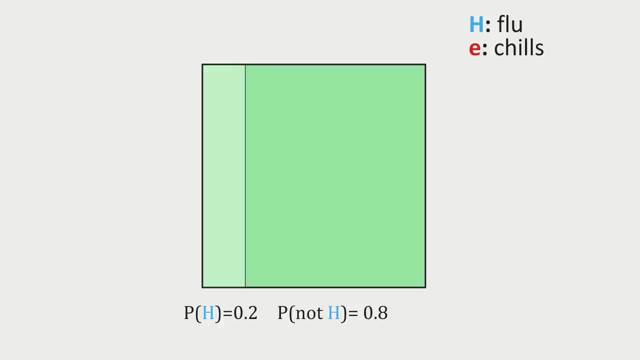 The other 80% doesn't. Now suppose that, given that someone has the flu, they're 90% likely to experience chills, And suppose that 20% of people who don't have the flu experience chills for other reasons. These numbers are made-up. they aren't the real-world. 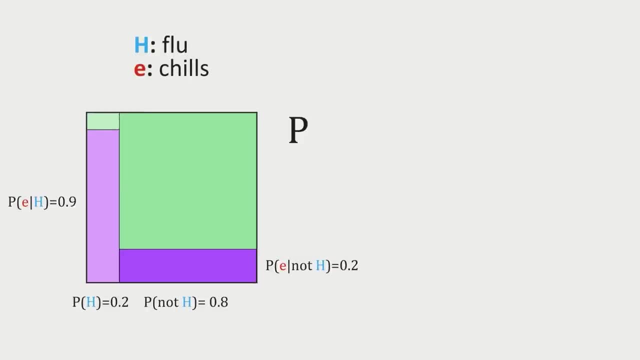 probabilities, Then if we want to estimate the probability that your friend has the flu, given the evidence that he has the chills, we must first observe that your friend is within one of these two rectangles, which together represent the total proportion of people who 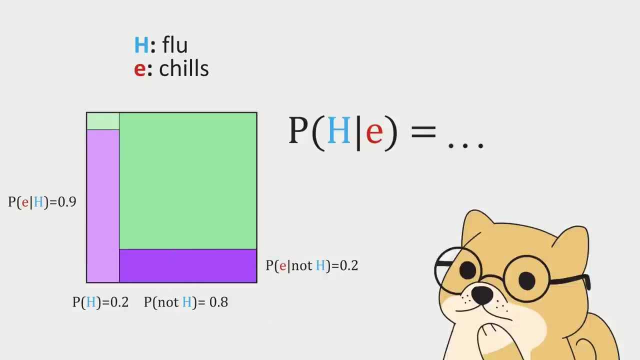 have the chills out of the general population. So we must calculate what proportion of people within these two rectangles have the flu, which is this rectangle out of these two rectangles added together. The proportion represented by this first rectangle is easily calculated by multiplying the. 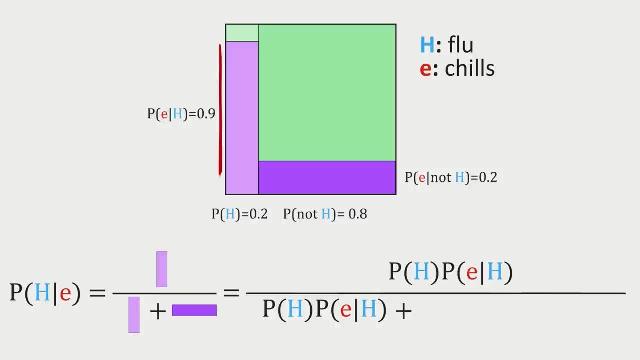 proportion of people having the flu by the proportion of people who have the chills, given that they have the flu. And the proportion represented by this other rectangle is calculated by multiplying the proportion of people who don't have the flu by the proportion of people who 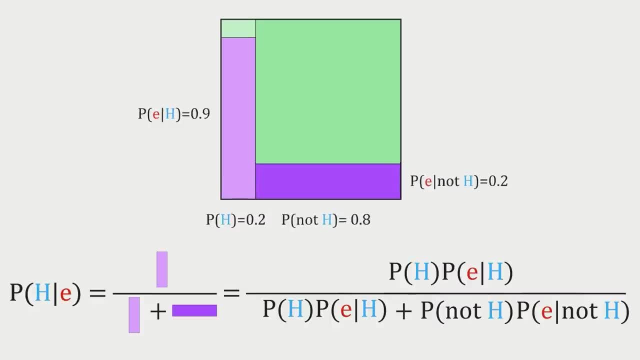 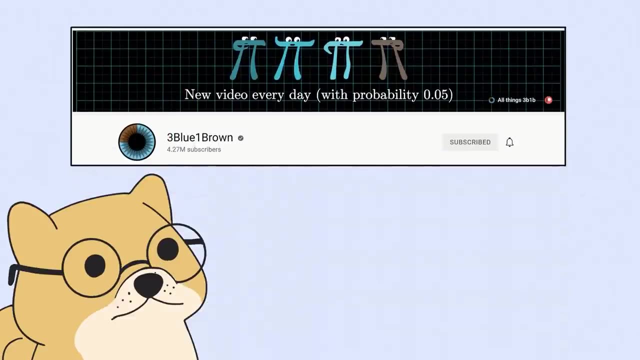 experience the chills. conditional on that, they don't have the flu. What comes out is Bayes' formula. This explanation with rectangles you just witnessed is how 3Blue1Brown explains Bayes' rule in his videos, But he explores these intuitions about 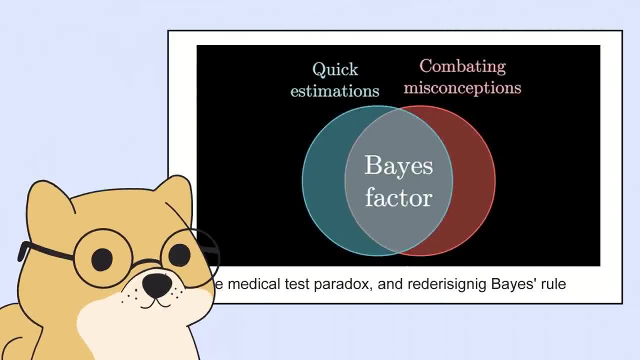 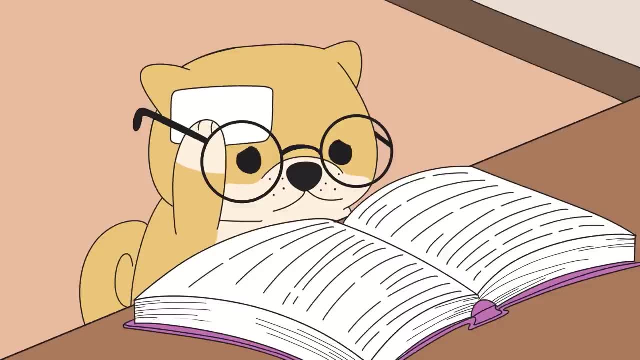 proportions to a much greater extent. so we suggest watching his videos about Bayes' rule. after finishing this one, We'll leave the link to his videos, plus other resources, in the video description. Using Bayes' rule for real problems can take some time to get used to. 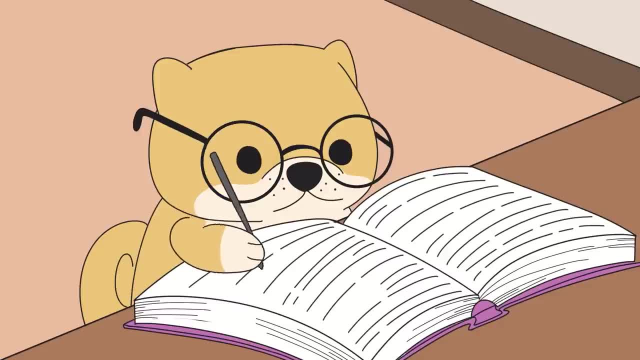 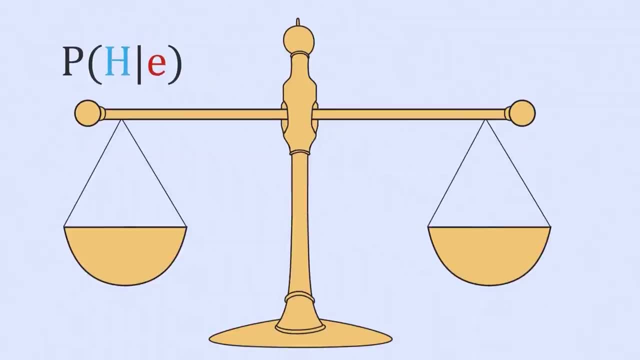 and you'll need to work through some examples to grasp it fully. But luckily there's an even simpler form of Bayes' rule which makes visualising the updating process easier Rather than directly telling you the probability of the hypothesis conditioned on the evidence. 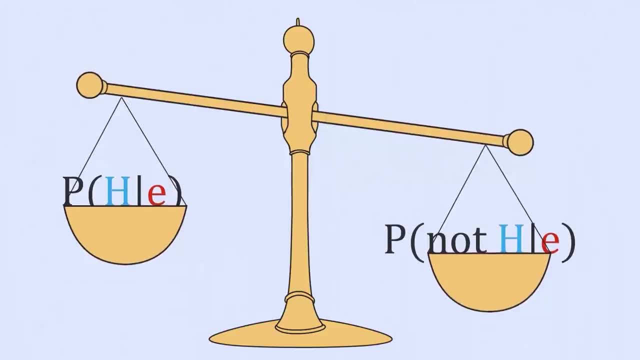 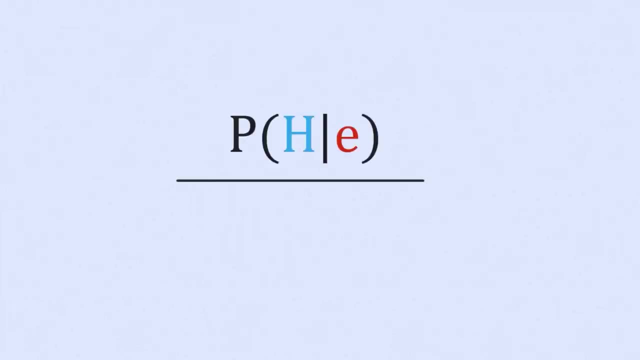 this form tells you how much more likely the hypothesis you're considering is compared to its negation after seeing the evidence. Therefore, we want to know the probability of the hypothesis conditioned on the evidence out of the probability of the negated hypothesis conditioned on the evidence. It's easy to calculate this. Just apply the. 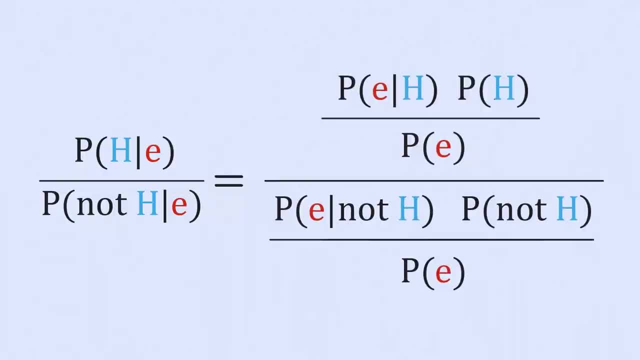 original formula to the numerator and denominator and we obtain this monster. But the probability of the evidence is the same for both updates. so it cancels out and you're left with this formula. Look at its right-hand side. There's a ratio of the priors and a ratio of. 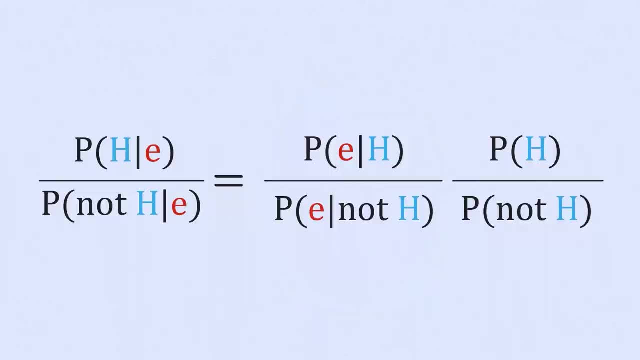 how well H and not-H fit the evidence at hand. Suppose that your prior probability for H is one third of your prior probability for not-H. Then you observe new evidence that is three times as likely under H than it is under not-H. Then H and not-H get updated to be exactly as likely. 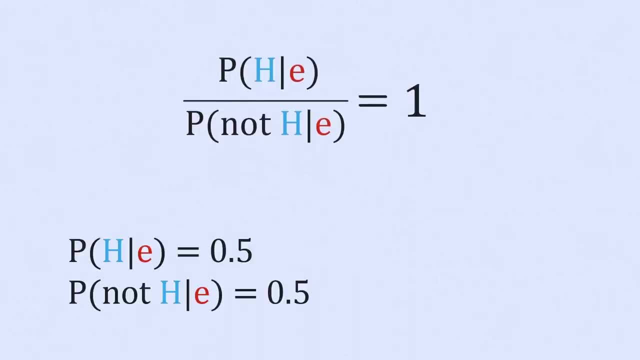 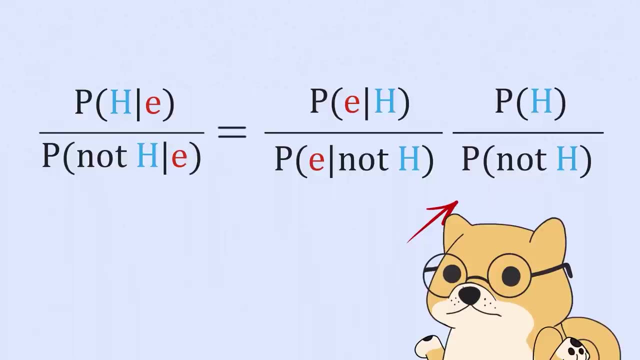 which means that H and not-H both have a posterior probability of 50%. See how these terms work together. The ratio of the priors is called prior odds because, well, the odds of the priors Odds are a slightly different way of representing prior odds than the odds of the prior odds. 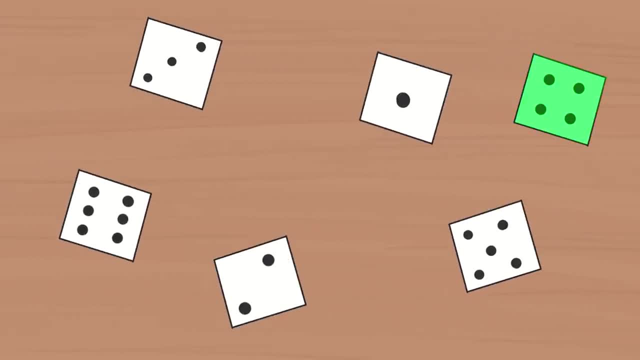 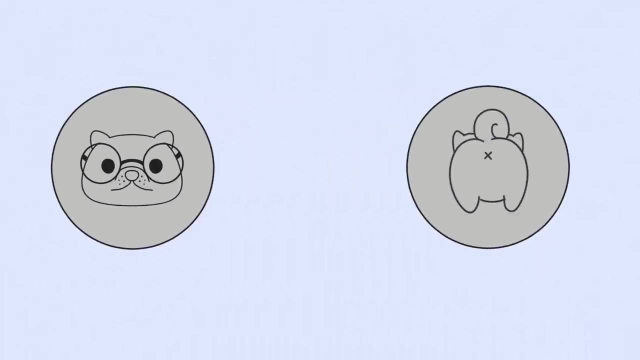 The probability that the toss of a die comes up to 4 is 1 out of 6.. The odds are 1 to 5.. The probability that a fair coin comes up heads is 50%, which corresponds to 1 to 1 odds. The prior: 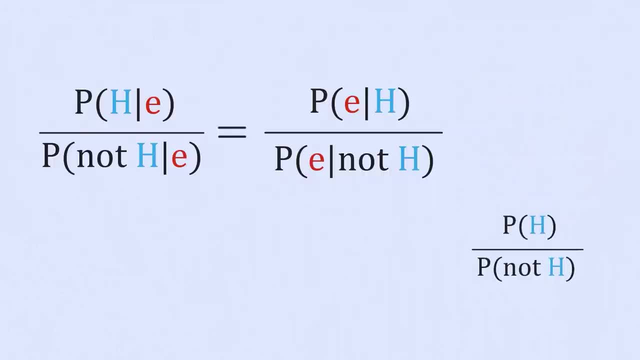 odds in this form of Bayes' rule are sometimes expressed with the notation O. The other factor is called the likelihood ratio, simply because it's the ratio of the likelihoods. It can be expressed with the notation L conditioned on H. The result is called posterior odds. 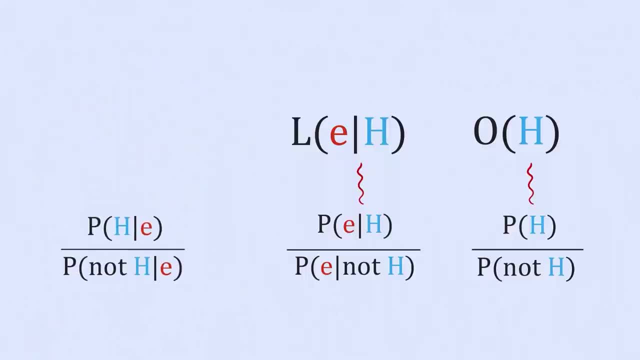 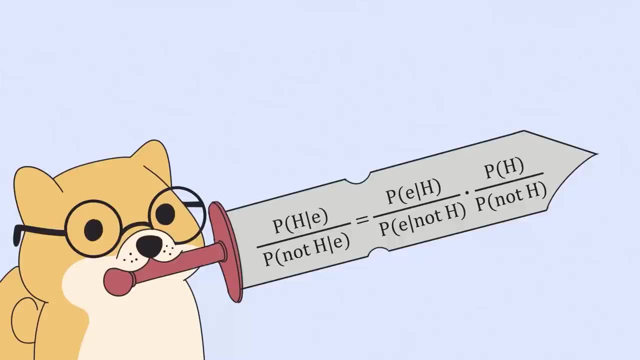 because well it represents the odds of the posteriors. It's often indicated with O conditioned on E, And this different way of expressing Bayes' rule is called the odds form of Bayes' rule. Now let's run through a real-world application of the odds form, taken from one of the pioneers. 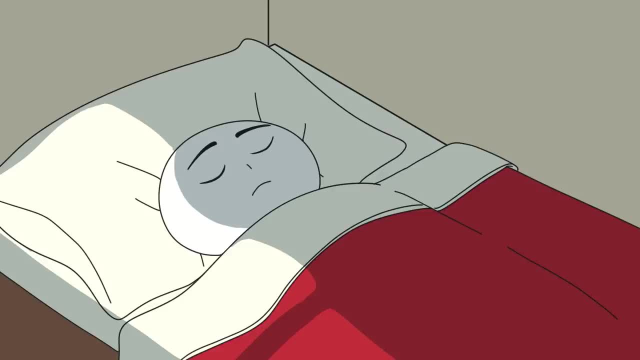 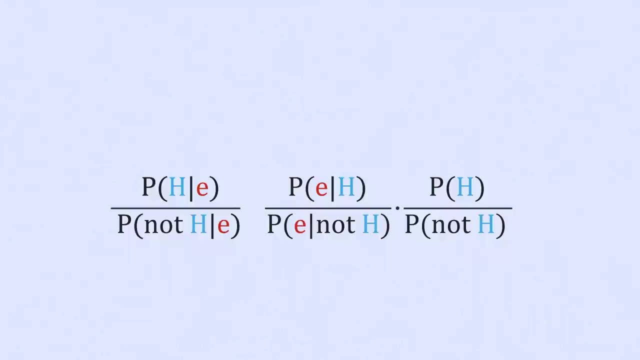 of Bayesian networks, Judea Pearl. You're awoken one night by the sound of your burglar alarm. You want to know the chance that your house is being invaded by a burglar or whether it's a false alarm. Let's apply the odds form. You know that if there's a burglary. 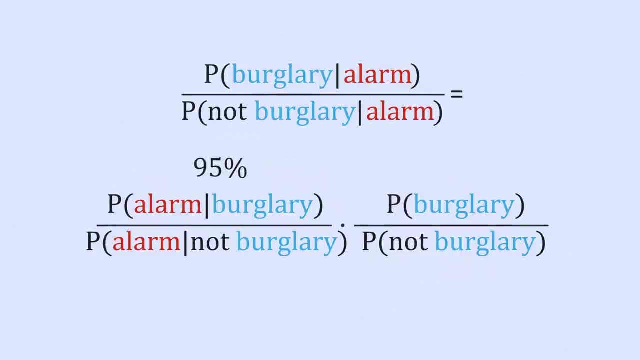 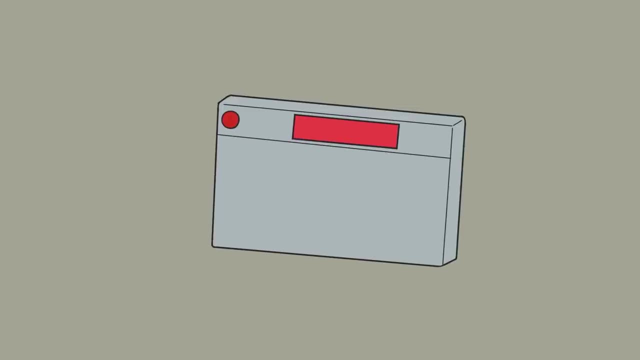 the alarm will go off with a probability of 95%. However, you also know, based on experience, that there's a one percent chance that your burglar alarm will go off even if there's no burglary. Sometimes it just malfunctions or there's a false trigger, like a tree. 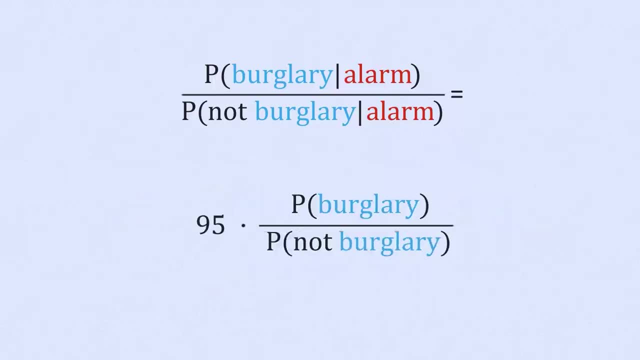 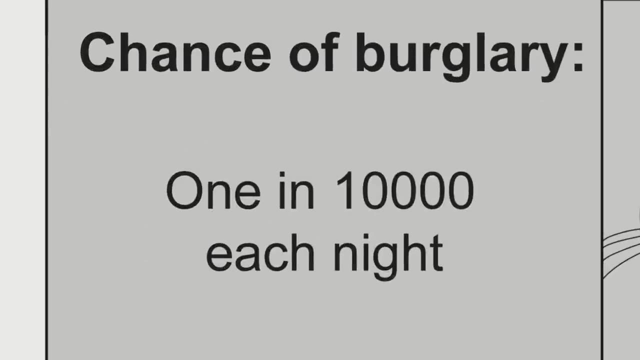 branch hitting your window. Therefore, the likelihood ratio is 95.. Finally, we know from local crime statistics that in your city there's about a one in 10,000 chance that a given house is burglarized each night, which means prior odds are 1 to 9,999.. Therefore, the posterior odds 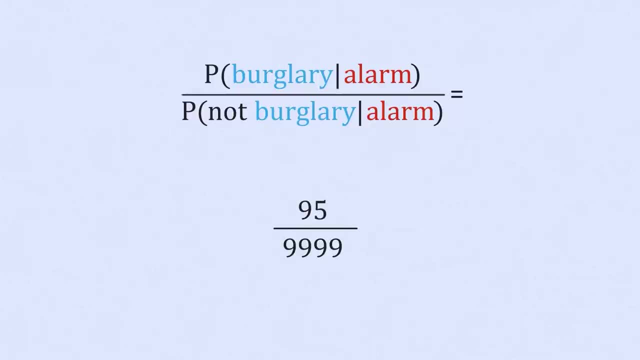 that your house is being burglarized are 95 to 9,999 after a burglary Number 3.. The probability of a burglary is one in 10,000.. The probability of a burglary is 1 to 9,999 after a. 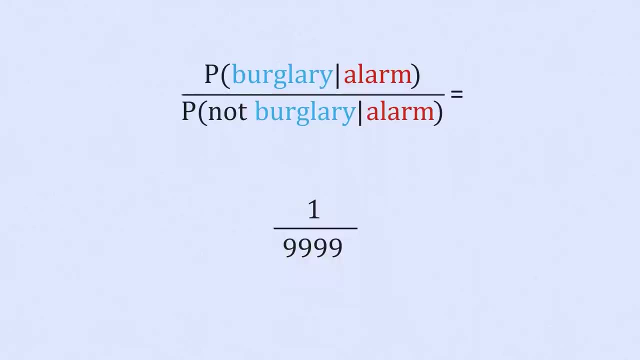 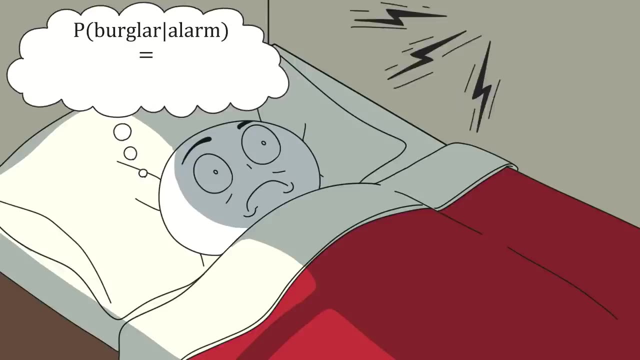 hearing the alarm, which correspond more or less to odds of 1 to 105.. This ratio equals 0.0095, which means that after hearing the alarm, the probability of your house being burglarized is 0.0095 times the. 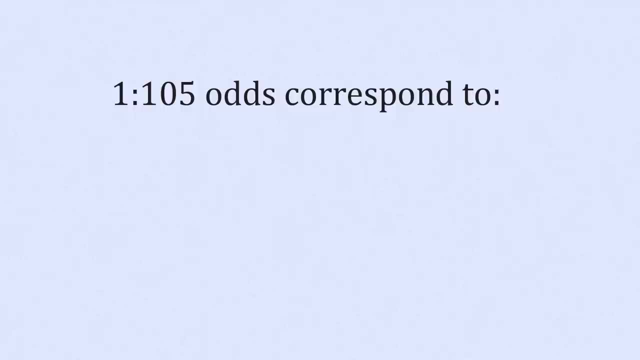 probability that your house isn't being burglarized. If we convert the posterior odds to probabilities, we get that the probability of burglary given alarm is 0.94%. That's almost 1%. Maybe a high enough chance to take the situation seriously, but not so high that you need to panic. It's worth reflecting. 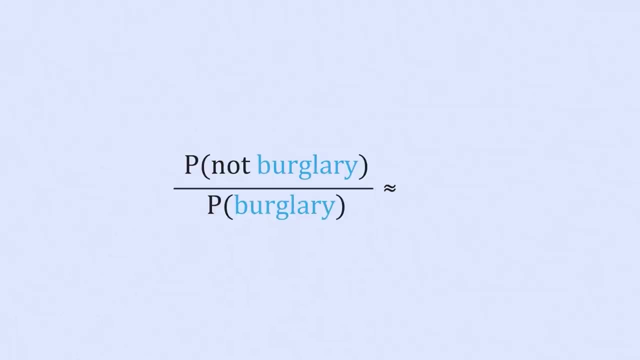 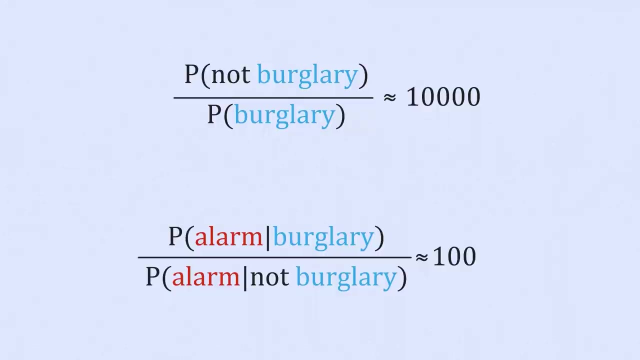 a bit more on this example. We started with the non-burglary hypothesis being around 10,000 times more likely than the burglary hypothesis, but the alarm was only around a hundred times more likely to activate in a world in which there was. 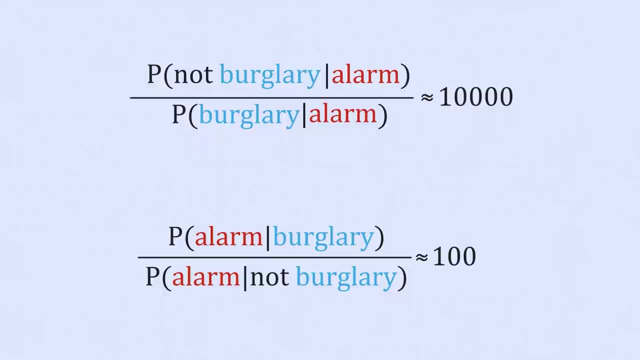 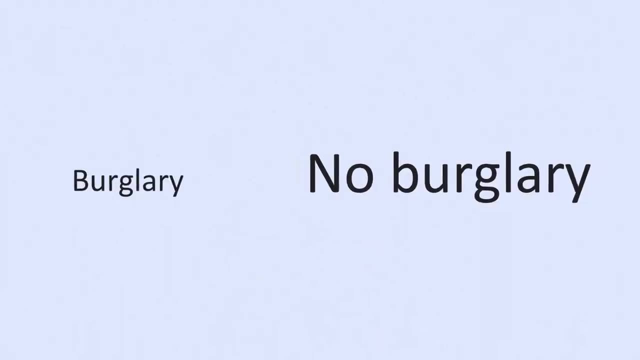 a burglary compared to a world with no burglary. This is only enough to cover two of the four orders of magnitude needed to tip the balance. The alarm going off makes the burglary hypothesis acquire credence relative to the non-burglary hypothesis, but only enough for the non-burglary hypothesis to 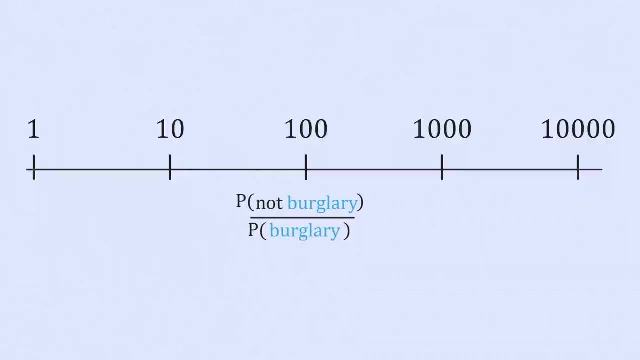 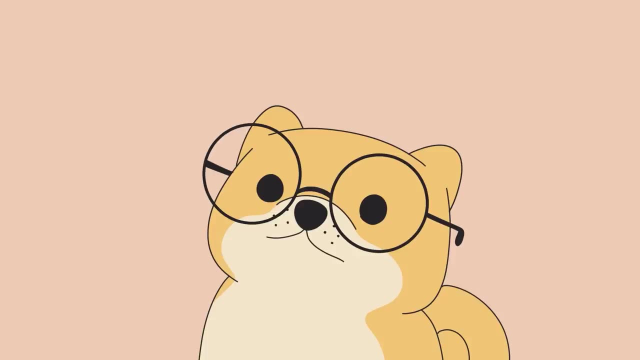 become a hundred times more likely instead of 10,000 times more likely than the burglary hypothesis. Even if you don't care to follow these calculations step-by-step, the important thing to understand about Bayes' rule is that in a simple equation we find the essence of how to change our beliefs in light of 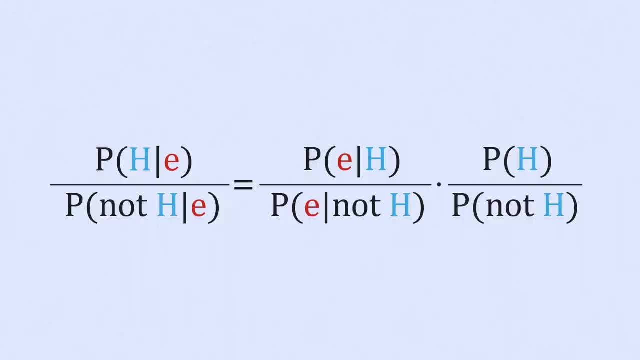 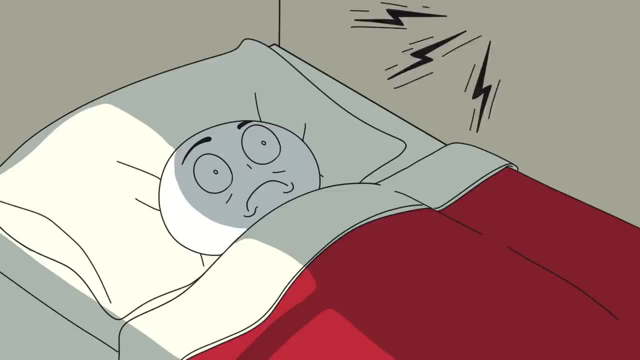 new evidence. In the odds form of Bayes' rule, we see that our updates are governed by multiplying our prior beliefs by the likelihood ratio dictated by evidence. Whenever we encounter new evidence, Bayesians ask us to consider what is the chance that we would have seen this evidence, if our theory is. 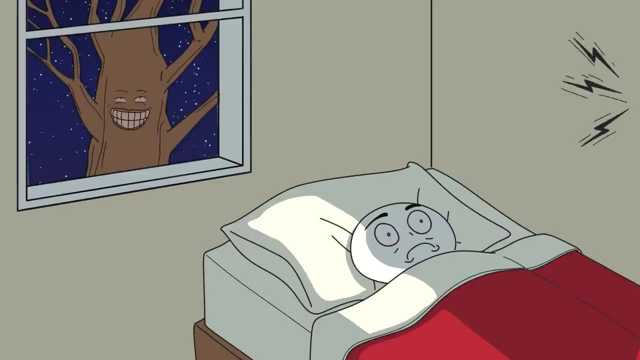 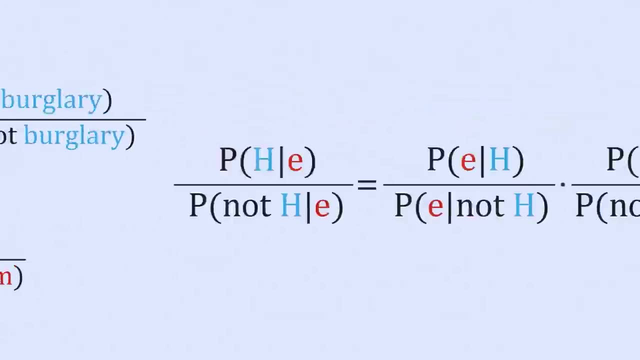 correct, and what is the chance of observing this evidence if our theory isn't correct? Multiplying this ratio by our prior odds gives us our posterior odds, what we should believe in light of the evidence. Now we'll consider one interesting implication of Bayes' formula. 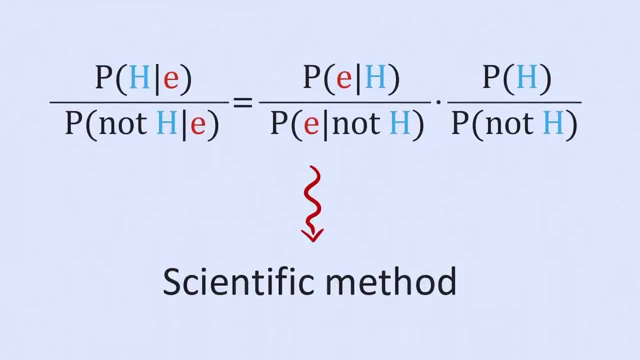 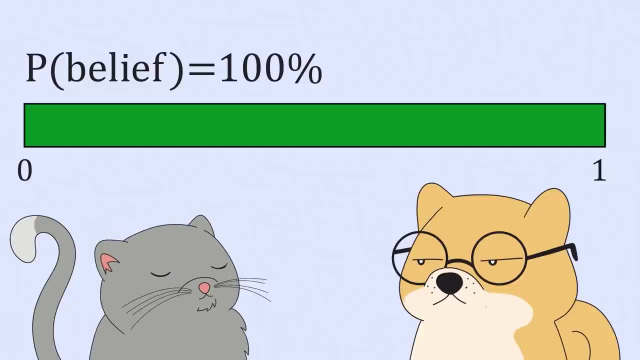 that you may recognize as a pretty central tenet of scientific reasoning. There are many more such implications and we'll probably flesh them out in future videos. Bayesians typically believe that we should never be absolutely certain in any of our beliefs, In other words, we should never assign a 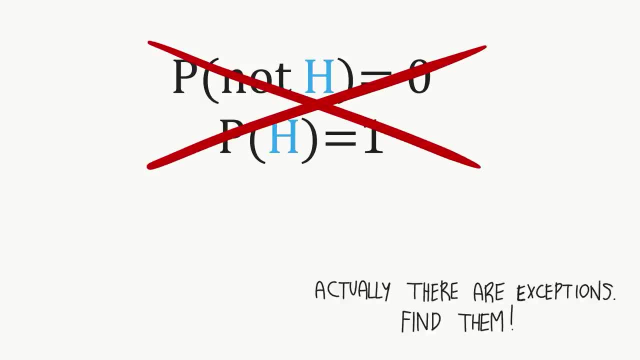 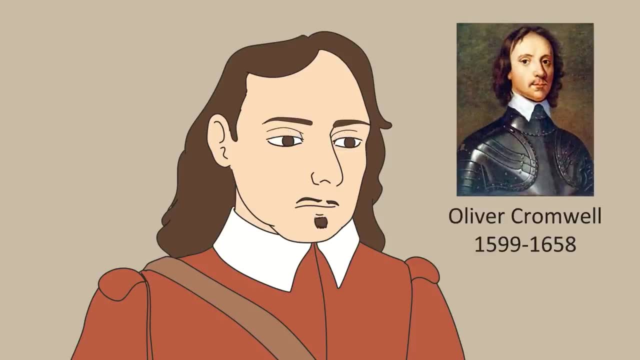 probability of exactly zero or one to any proposition, no matter how absurd. This idea is sometimes called Cromwell's rule, named after the English scientist, statesman Oliver Cromwell, who once declared to the General Assembly of the Church of Scotland: I beseech you in the bowels of Christ, think it possible. you may be mistaken. 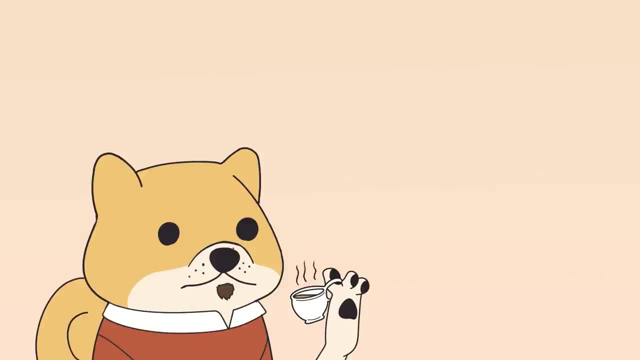 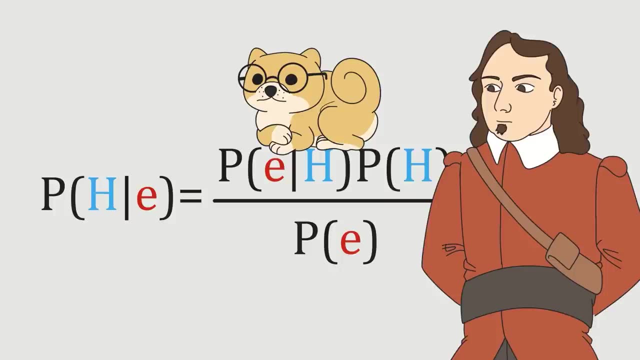 The rationale for Cromwell's rule can be readily seen by asking what would happen if we ever assigned 100% or 0% confidence to any of our beliefs. Let's look at the original form of Bayes' rule again. Let's say that you think the 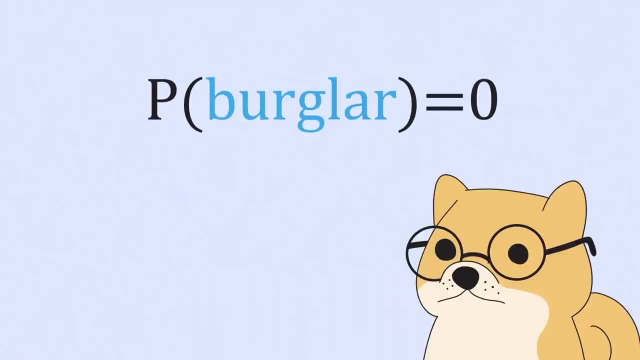 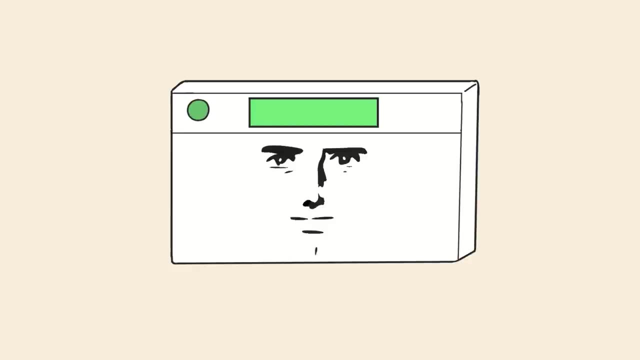 chance of your house getting burglarized is exactly zero. You've never even heard of a burglary happening in your city. Burglaries- What even are they? Also, this time we have an extremely accurate alarm. The chances of it having an error are one in a trillion. It will only signal. 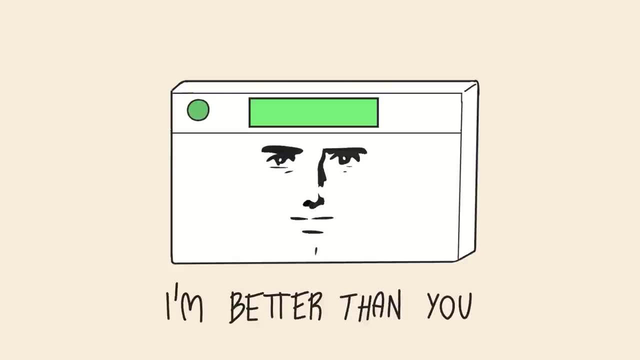 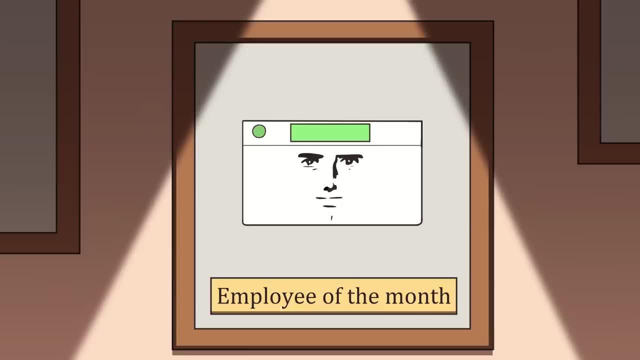 a false alarm on one in every trillion nights, or about once every 273 million years, And in only one in a trillion burglaries will it ever fail to warn you, Even though the alarm is extremely good at its job. Bayes' rule tells us that hearing. 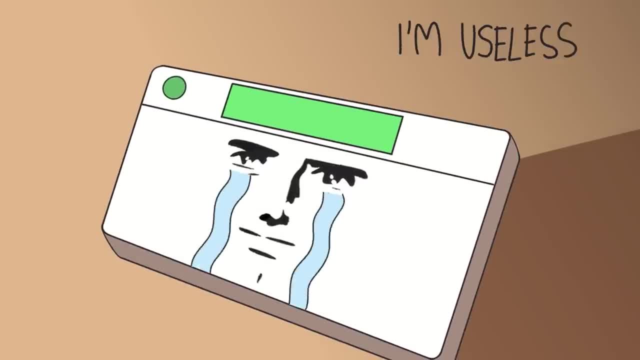 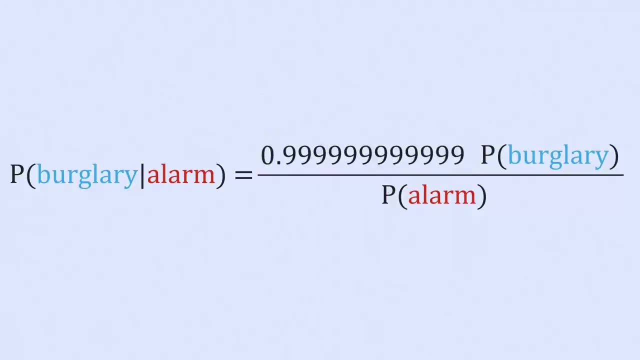 the alarm provides precisely zero update to your prior belief about being burglarized. Here's why, In the numerator, we have P, which in this case is extremely high, multiplied by the prior probability. However, the prior probability of a burglary is zero. remember, If we multiply these two, 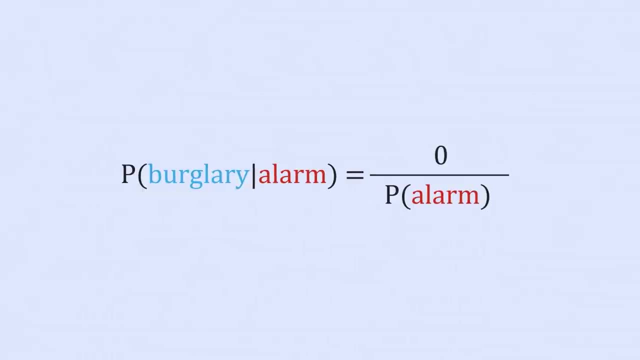 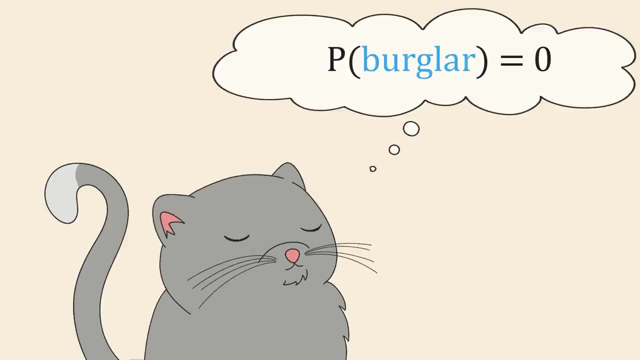 quantities in the numerator, we get zero. And we know that if the numerator is zero, it doesn't matter what's in the denominator: the result must also be zero. So in other words, your total and resolute certainty that you're not being burglarized. 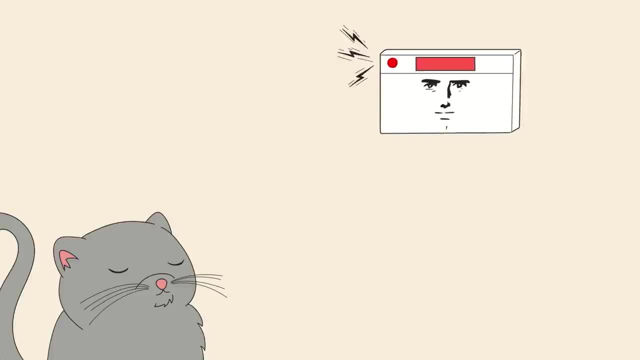 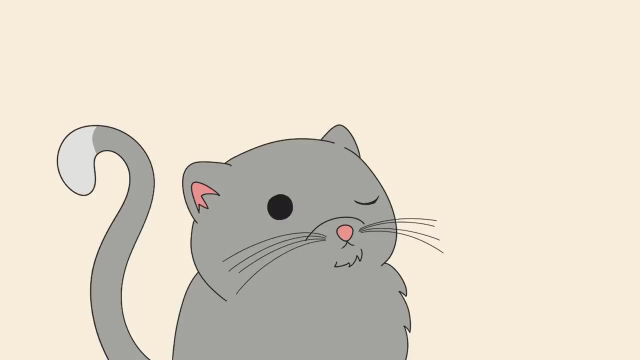 was completely unshaken by the evidence, Even in the presence of an extremely ludicrously reliable alarm. your faith is unfazed, And that's kind of a problem, right? Wouldn't you at least want to doubt your initial hypothesis a tiny bit? 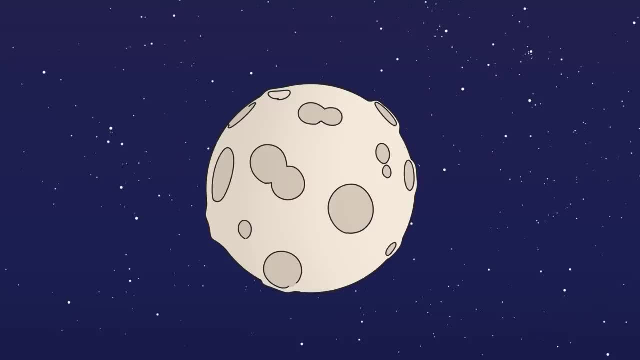 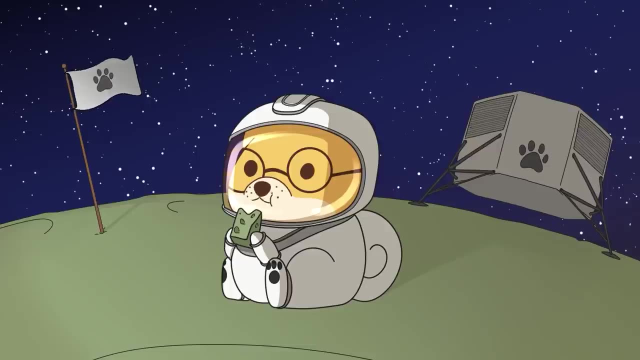 As Bayesian statistician Dennis Lindley put it, you should always leave a little probability for the moon being made of green cheese. It can be as small as one in a million, but have it there, since otherwise an army of astronauts returning with samples of said cheese will. 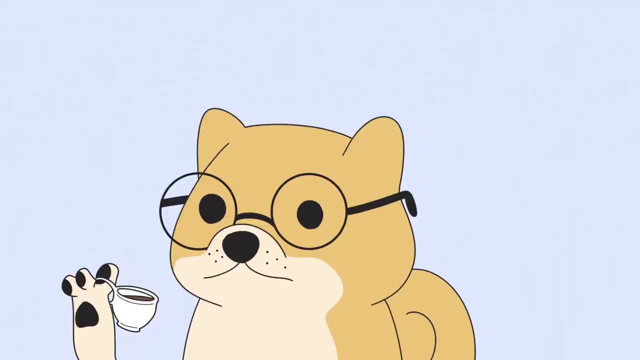 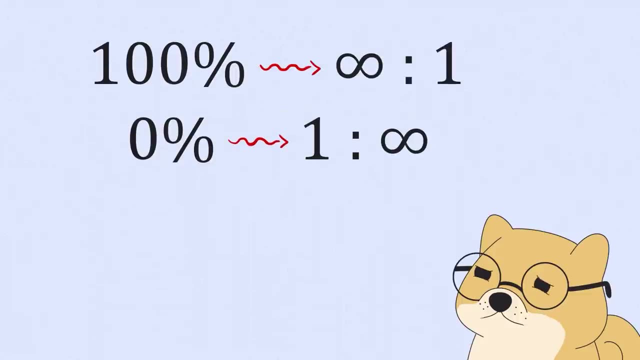 leave you unmoved. Another way of thinking about this is in terms of odds. A probability of 100% or 0% corresponds to odds of infinity, to one, or one to infinity, which is kind of strange. You've never observed infinite evidence, so it doesn't make sense to have infinity. 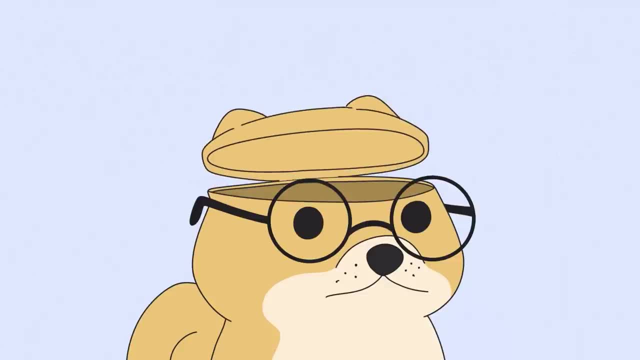 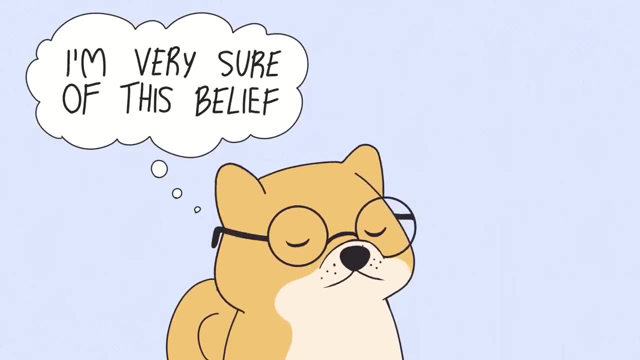 For Bayesians, Cromwell's rule is just a generalization of the idea that we should be open-minded, We should be ready to change our minds about anything and, in theory, some amount of evidence should be sufficient to drive our beliefs in the other direction from. 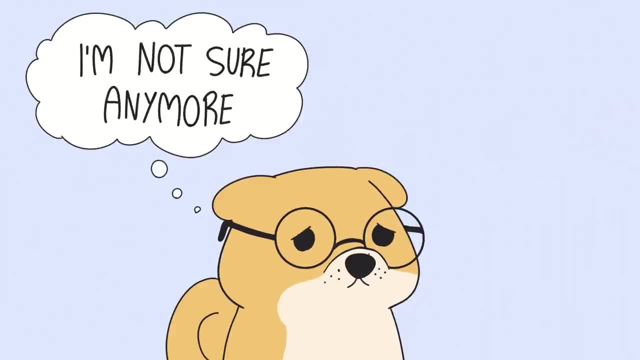 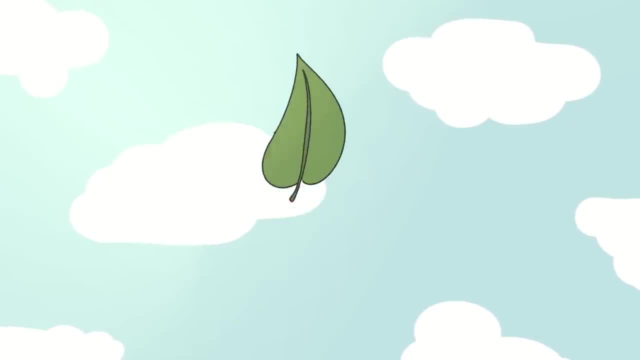 where they are now, no matter how confident we happen to be at the present moment. More generally, Bayesians see beliefs as a way of building an understanding of the world. The Bayesian view of evidence tells us that our beliefs should dance like a leaf in the 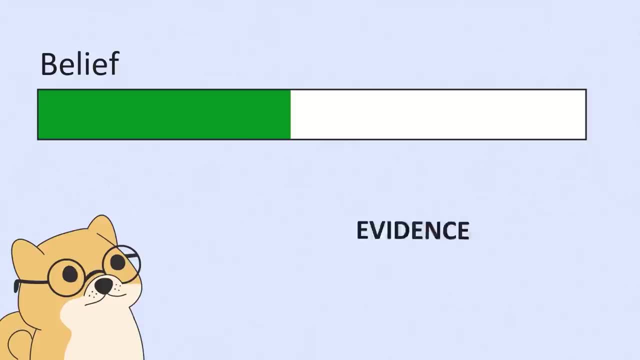 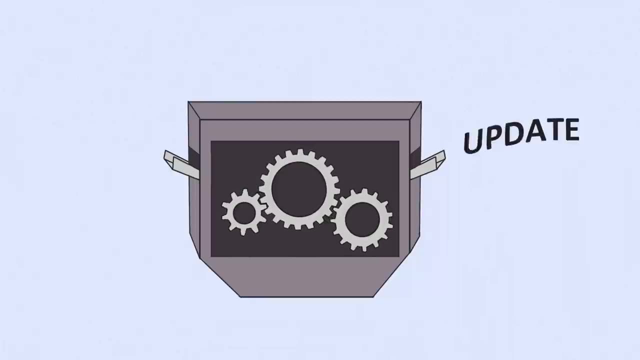 wind drifting. in whatever way the evidence pushes them Truly, adopting Bayesian reasoning is striving to change our beliefs, the exact right amount in the face of new evidence. Bayes' rule is more than just a formula. It's a precise rule for reasoning, Much like 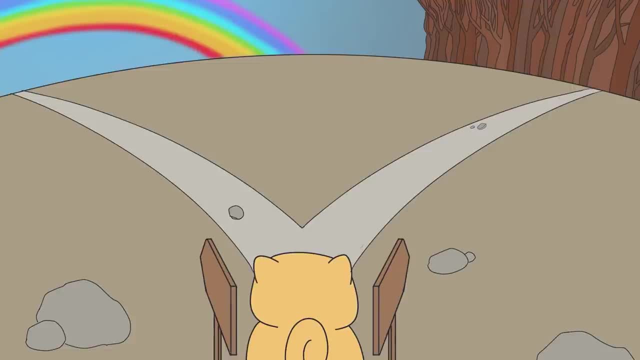 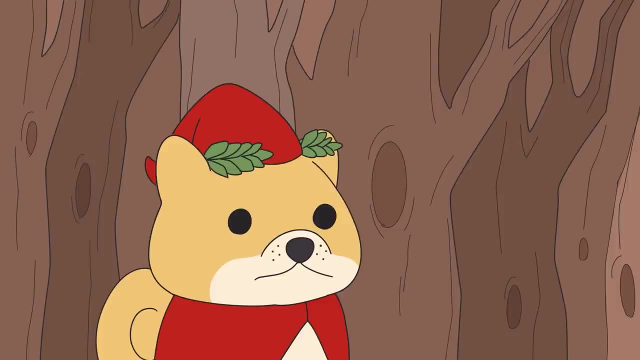 how. the laws of physics govern how the universe works. laws of human understanding govern how we should pursue truth, and no one is exempt from them. If you choose to ignore them, your journey to the truth will be hindered. Of course, Bayesians don't claim that we can realistically follow these calculations. 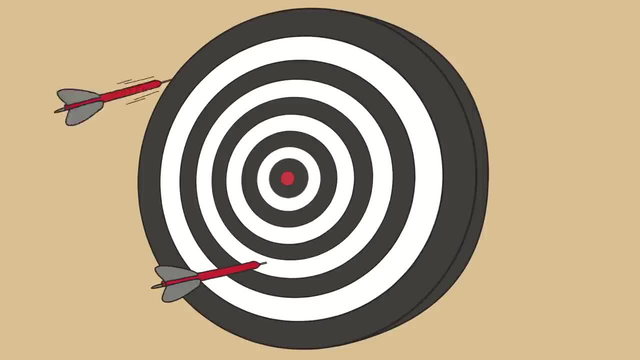 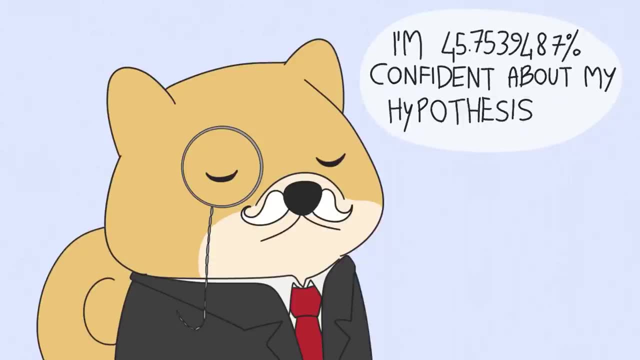 for all of our beliefs. Nailing down the precise likelihood ratio for real-world evidence might be extremely tough. It's important not to make the mistake of pretending that we can be more exact than is possible by asserting extreme confidence in specific numbers, especially in cases when the numbers only serve to elucidate our subjective impressions. 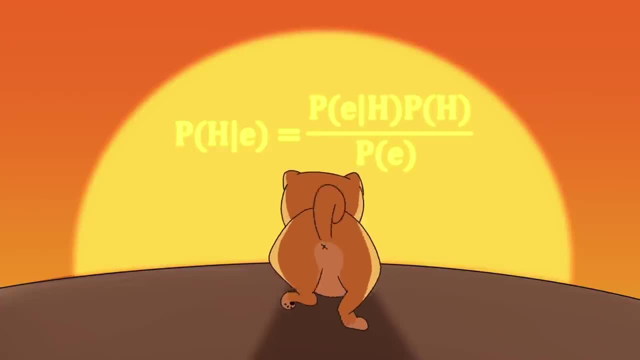 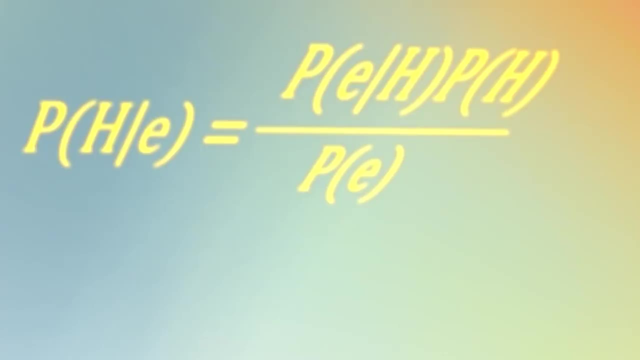 which might be wrong. But even with these caveats, Bayes' rule means that there is a precise and general method for changing our minds, And even just knowing that a method for arriving at truth exists should inspire us to approach it. If we reach towards this,